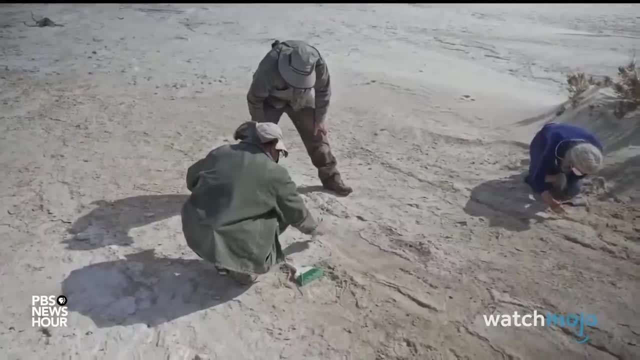 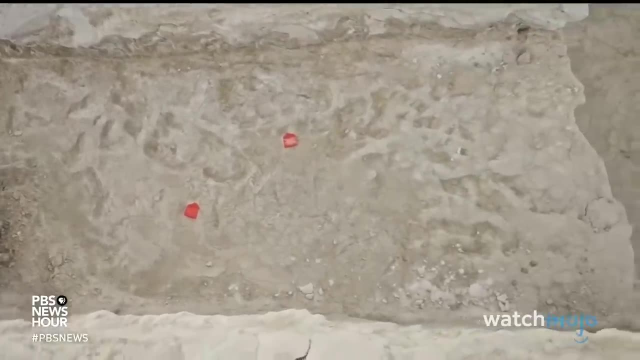 Columbia, Canada, that dated back about 13,000 years. At the time, these were the oldest footprints discovered in the world. These footprints are believed to have been found in North America, But just a few years later- in 2021, that record was shattered. 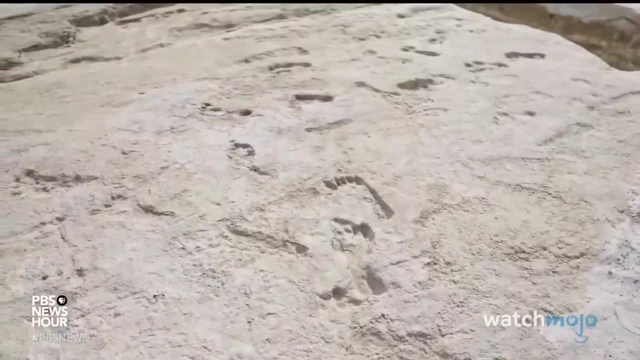 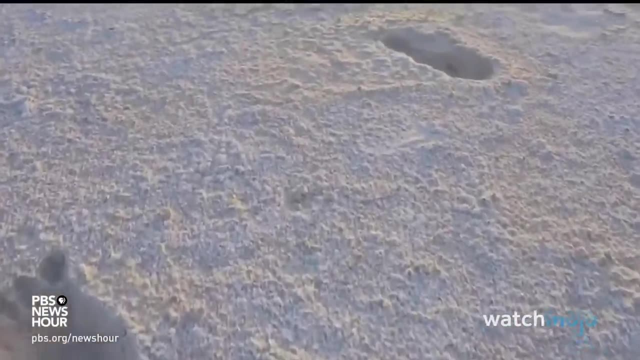 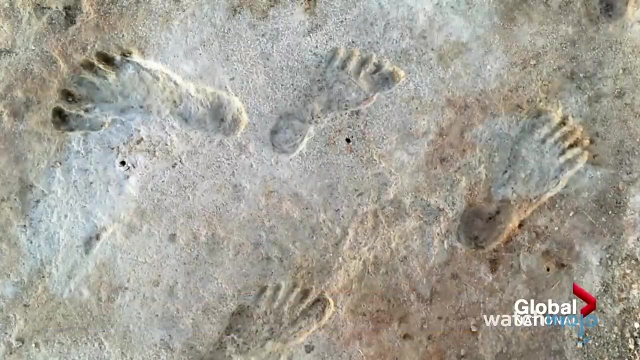 The footprints show how humans coexisted with large wild animals. Many are of children and reveal a story about everyday life and play. Archaeologists working in New Mexico's White Sands National Park unearthed tracks that are between 21,000 and 23,000 years old. 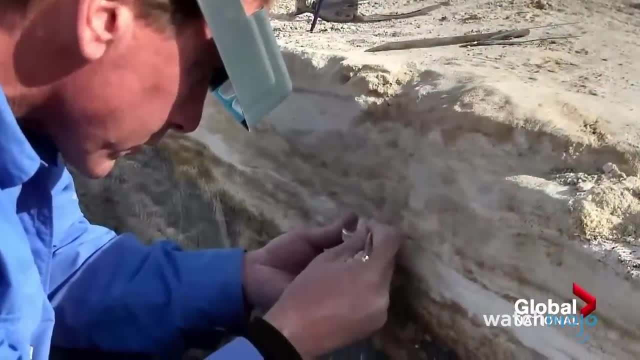 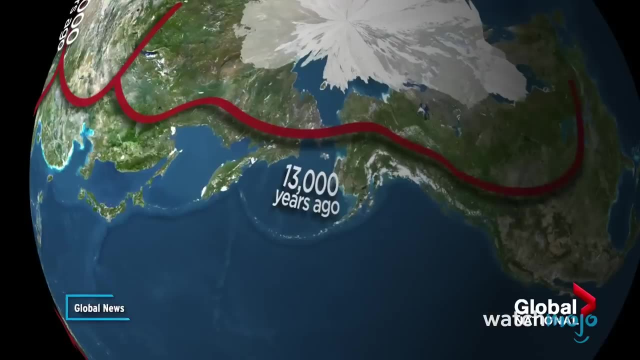 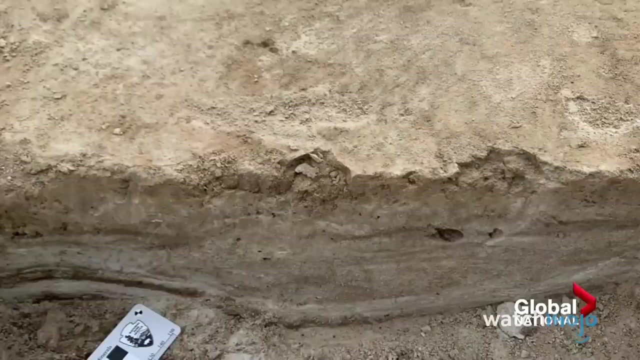 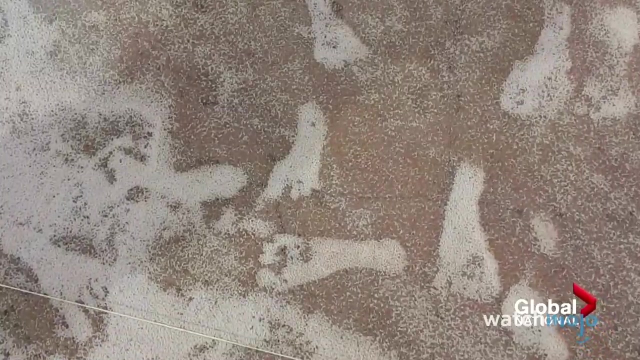 Not only does this almost double the record for oldest footprint in North America, it also completely restructures our understanding of early North American settlement. Prior to this game-changing discovery, most experts dated the continent's earliest habitation to between 11,000 and 13,000 years ago. 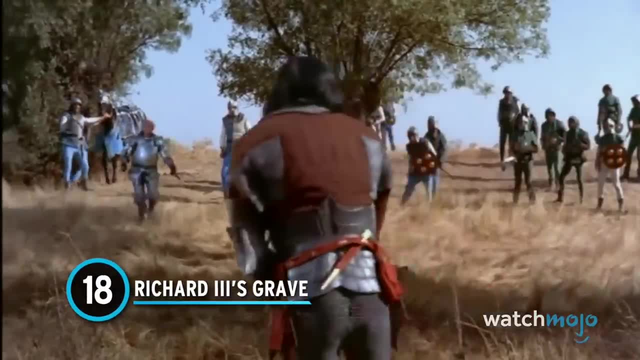 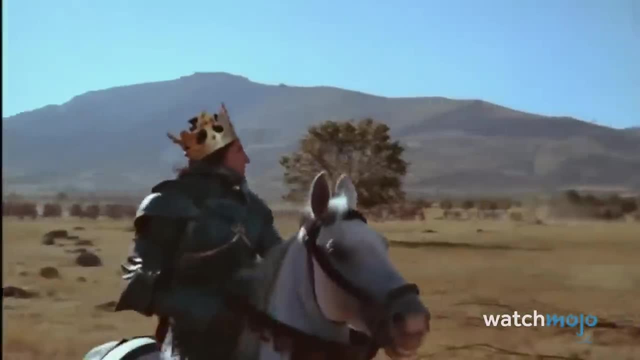 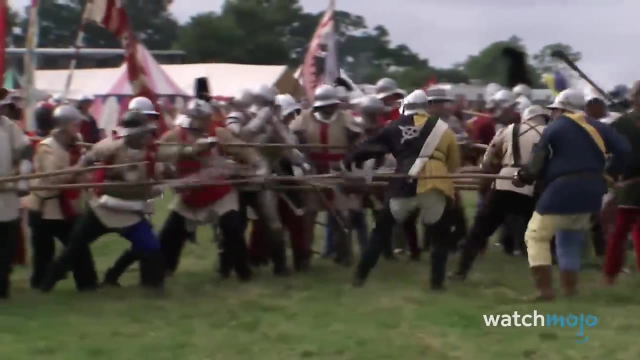 18. Richard III's Grave. This controversial figure ruled as King of England and Lord of Ireland until 1885, when he died in the Battle of Bosworth Field. With his death, the Wars of the Roses came to an end and with it the Middle Ages in England. His reign was later immortalized in Shakespeare's 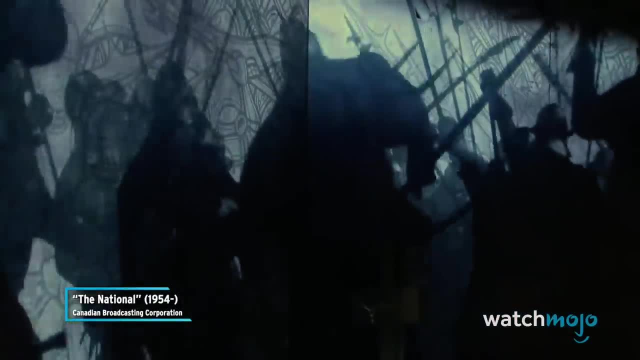 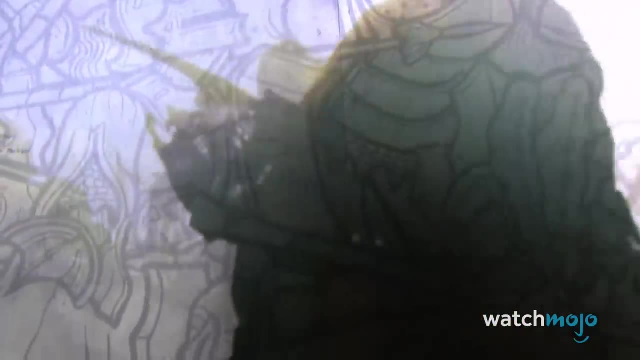 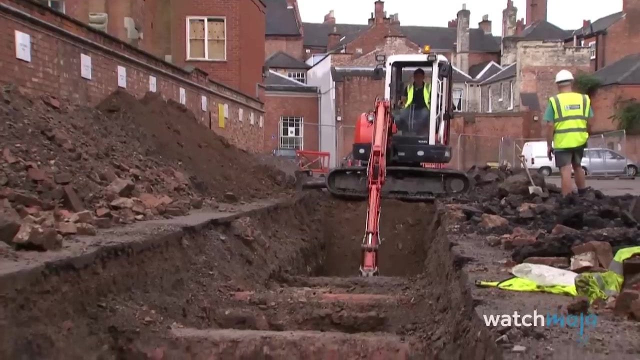 eponymous play. As Shakespeare put it, my kingdom for a horse, But Richard had lost his steed in battle and he fell dead on the ground, The last British king to die on the field of battle. 19. Richard III's Death. Following Richard III's death: his. 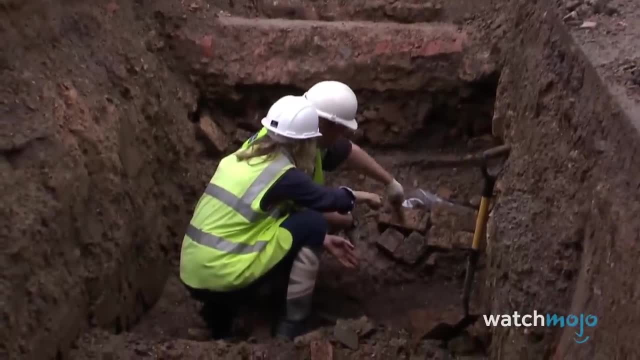 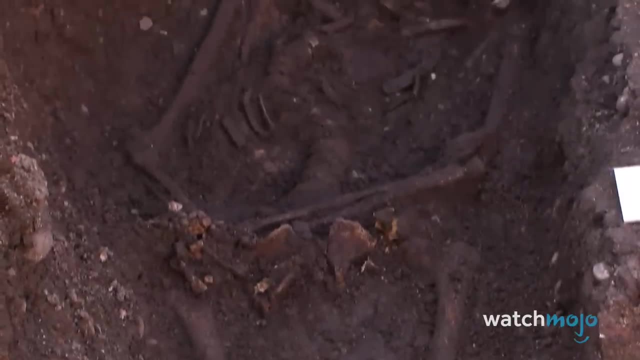 corpse was quickly buried and lost to time Until 2012.. That year, researchers discovered the foundations of a medieval church underneath a modern parking lot, and it was there that they found the skeleton of Richard III, But this is where he was discovered. 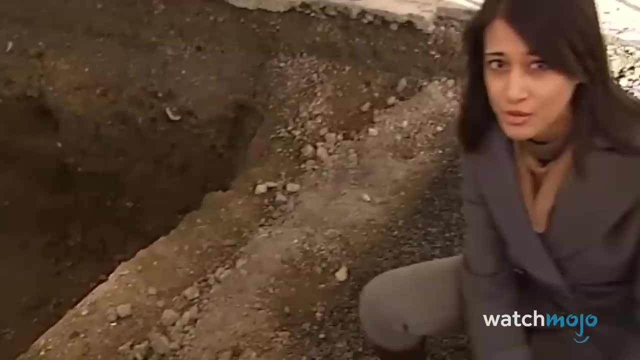 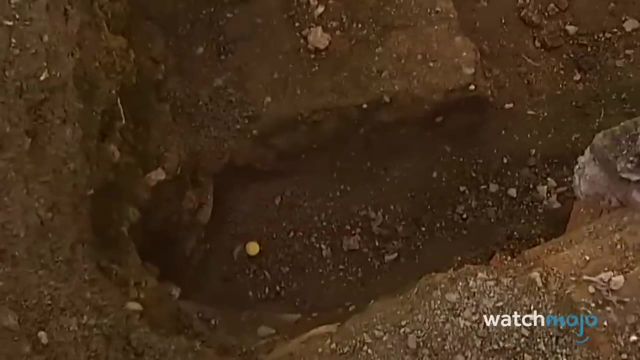 His well-preserved skeleton was buried without a coffin or a shroud. A combination of markings on the bones and genetic analysis proved what the experts had hoped for: After more than 5 centuries, we had finally found one of England's most notorious rulers. 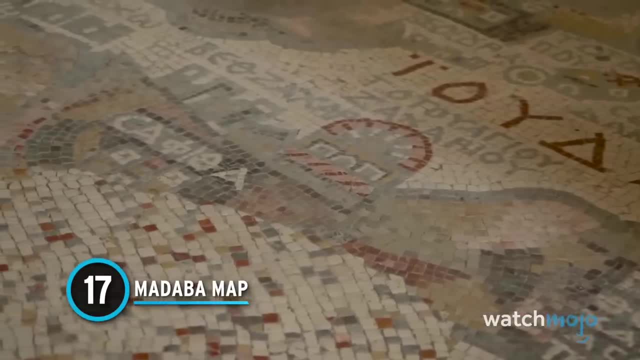 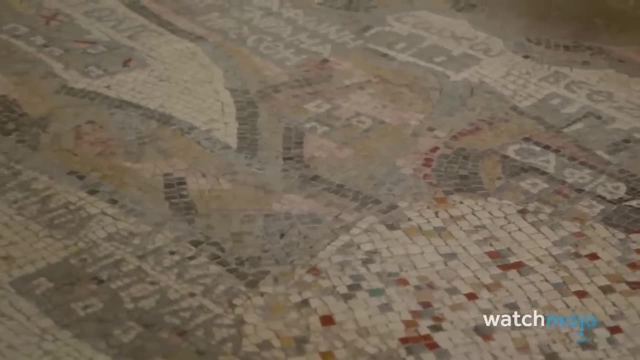 17. Madaba Map. In the late 19th century, construction began on a new Greek Orthodox church in Jordan's capital city of Madaba. While building the new structure, workers unearthed an ancient mosaic on the floor of the existing church. 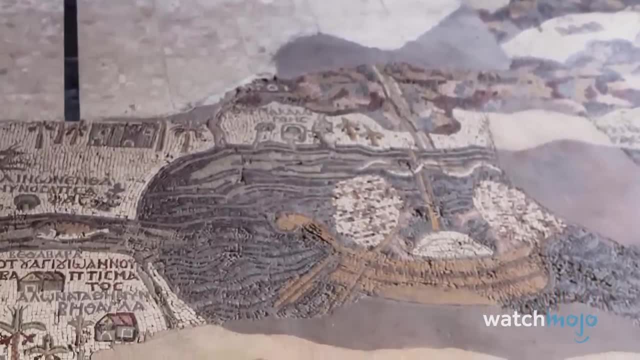 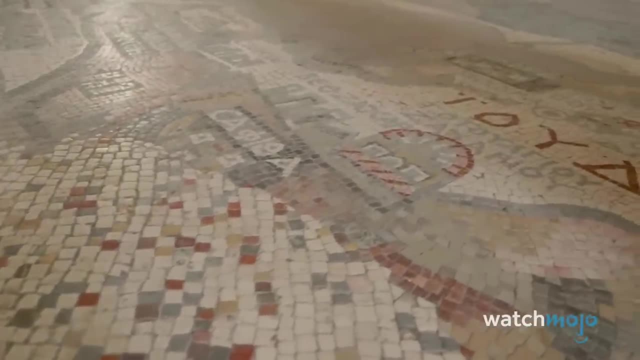 This mosaic is now known as the Madaba Map, and it shows parts of the Middle East Dating to the 6th century. the map contains the oldest known depiction of both Jerusalem and the Holy Land. Not only that, but it was used extensively to locate sites mentioned in the Bible. 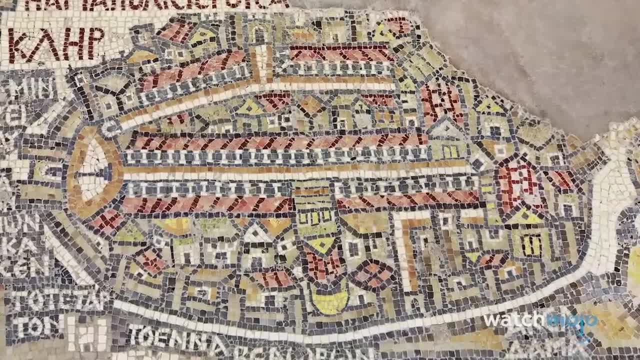 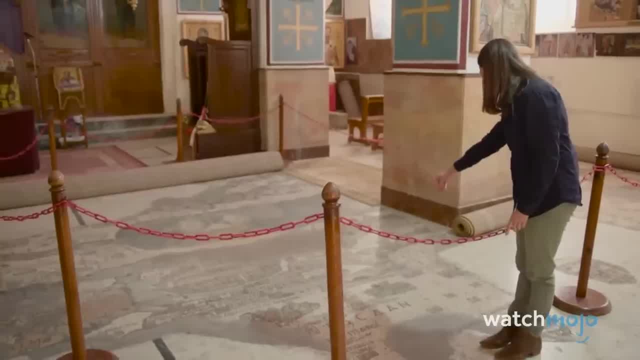 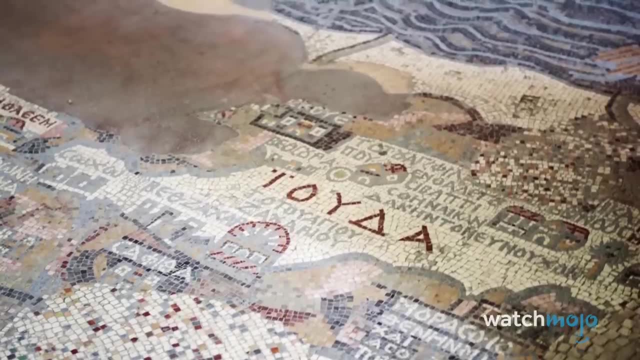 and it is currently the oldest geographic floor mosaic in the world. But also, if you look, you'll see other cities. We have Jericho here, we have Ascalon and Gaza here, Right at the top, you'll see the Dead Sea. 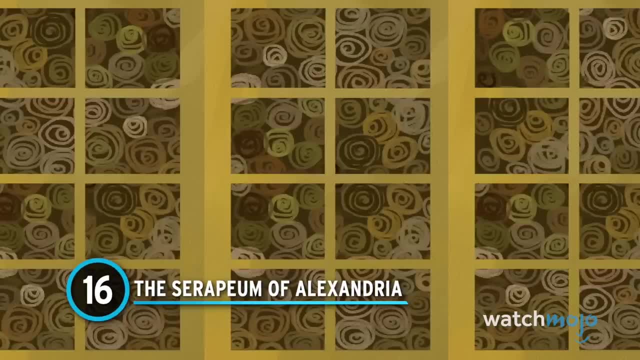 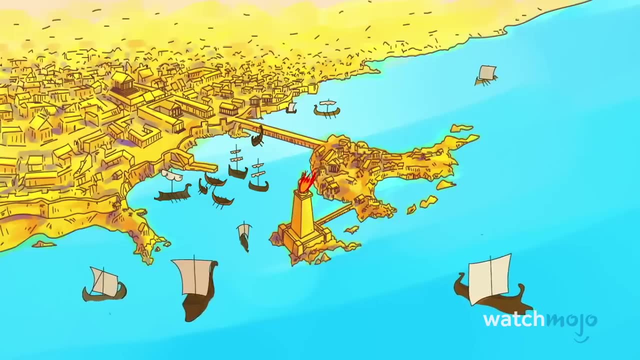 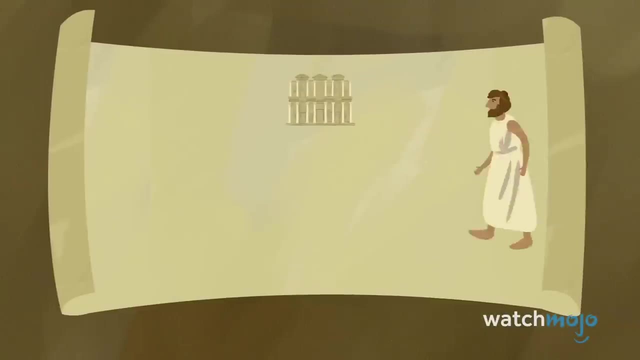 16. The Serapium of Alexandria, Serving as the greatest library of its age. the Library of Alexandria attracted scholars to Egypt and served as the ancient world's symbol of knowledge. In its prime, the Library of Alexandria housed an unprecedented number of scrolls and attracted some of the Greek world's greatest minds. It proved so popular that a so-called 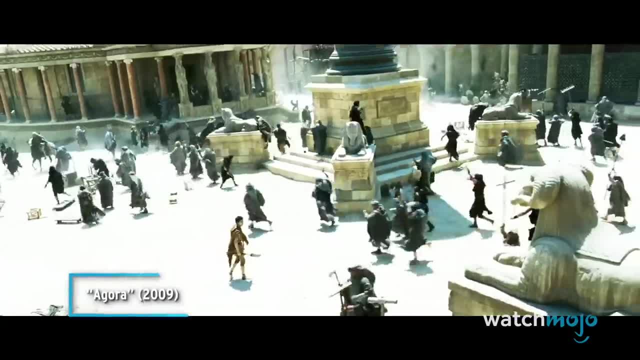 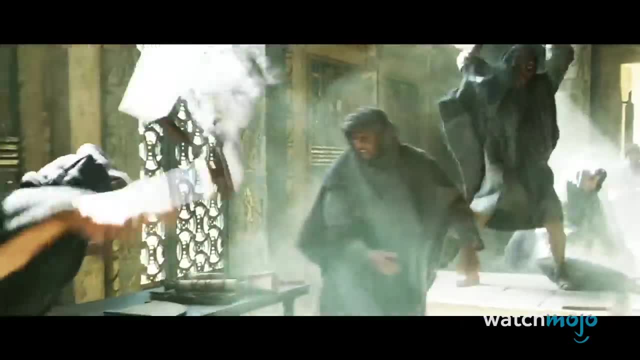 daughter library was built on the site of the ancient Greek library. The library was built on the site of the Serapium of Alexandria. The Serapium lasted a bit longer than its famous father and it was finally destroyed in the year 391.. The site later became a Muslim cemetery In the 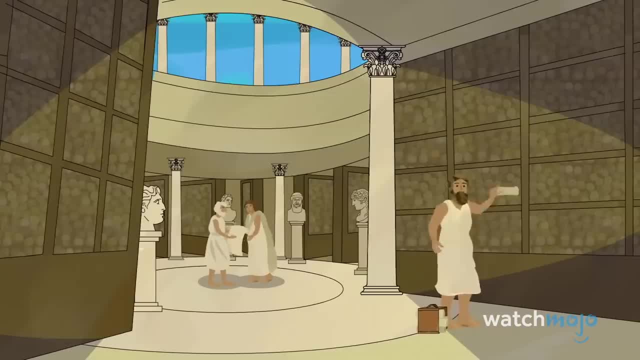 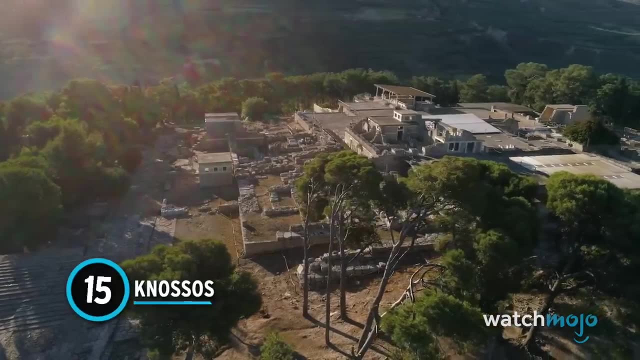 mid-1940s, the foundations of the Serapium were discovered And with it one of the greatest centers of learning in human history was unearthed. 15. Knossos, Found on the Greek island of Crete, Knossos is often regarded as the oldest city in Europe. And that's saying something- Featuring a massive and world-renowned palace complex. Knossos was the primary capital of the ancient Minoan civilization, which inhabited both Crete and other Aegean islands. 15. The Serapium of Alexandria. 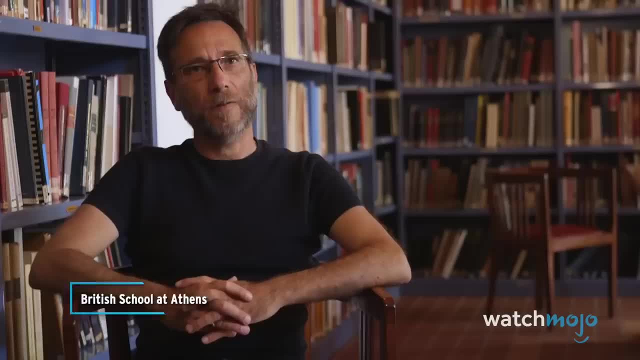 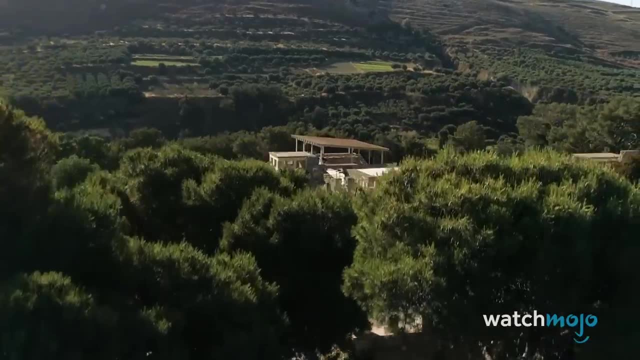 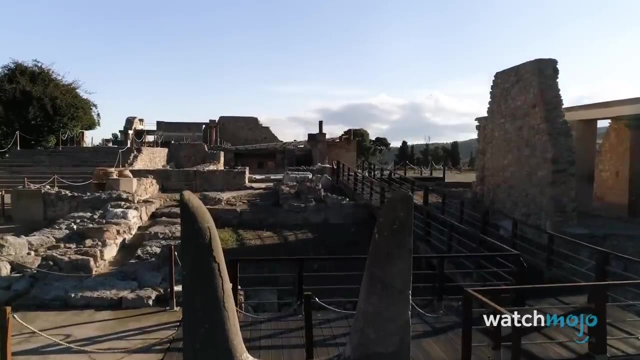 However, very few know that around the palace there was a very extensive settlement, the largest urban center in Crete and mainland Greece. 16. The Serapium of Alexandria. The civilization prospered from about 3500 BCE to 1100 BCE, But it's believed that Knossos had been inhabited since the Neolithic. 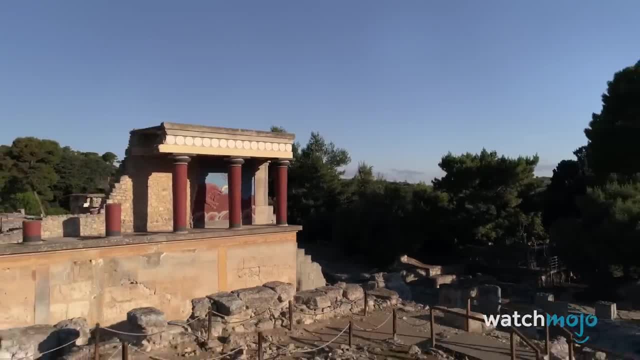 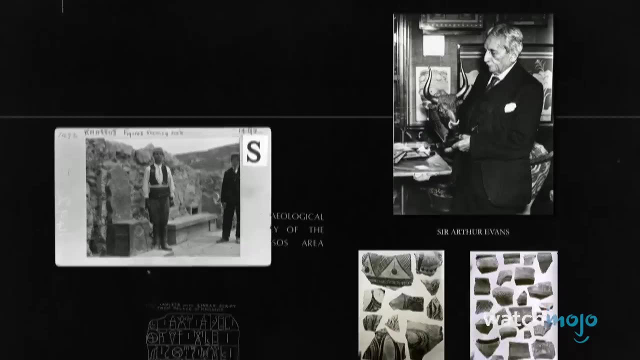 period 17.. The Serapium of Alexandria and the Serapium of Alexandria were built on the site of the Neolithic period. An amateur archaeologist named Minos Kalokirinos discovered the location of Knossos in 1878, and the ancient site was unearthed by Sir Arthur Evans throughout much. 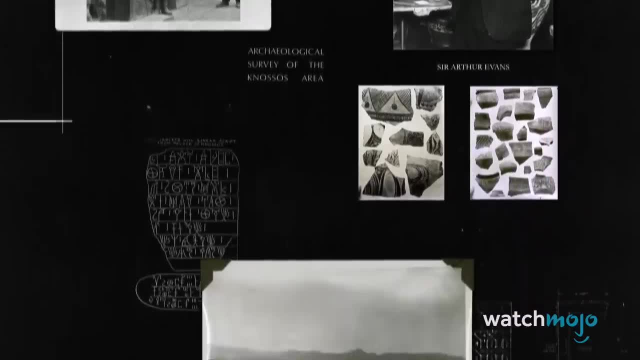 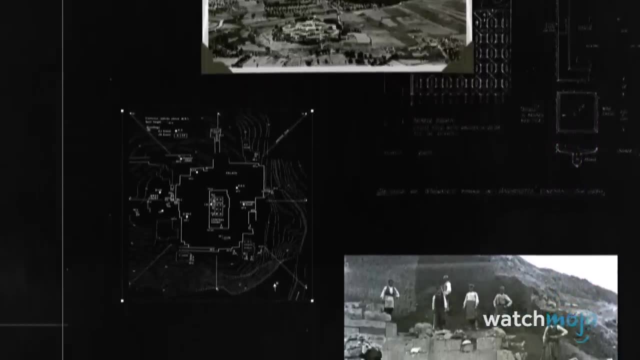 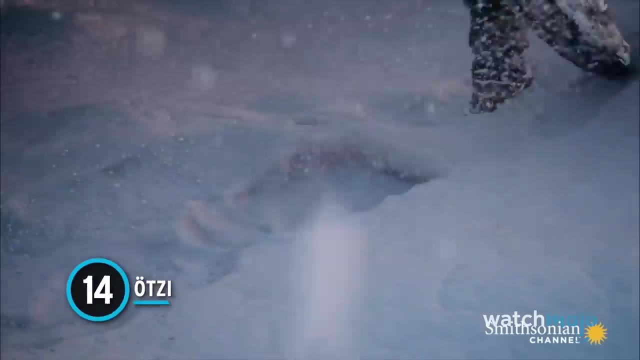 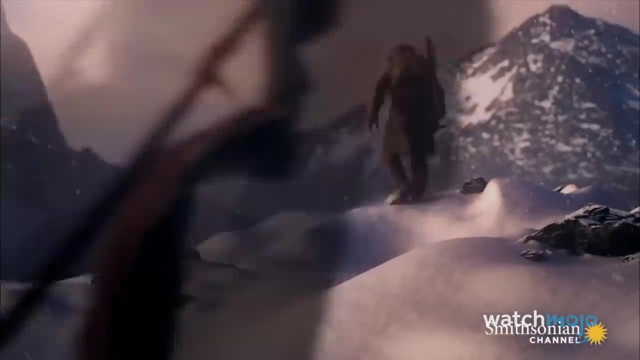 of the early 1900s, 14. Ötzi. Just imagine Mount Mountaineering through the Alps when you stumble across an ancient human corpse embedded in a glacier. This is exactly what happened to German tourists Helmut and Erika Zeman in September of. 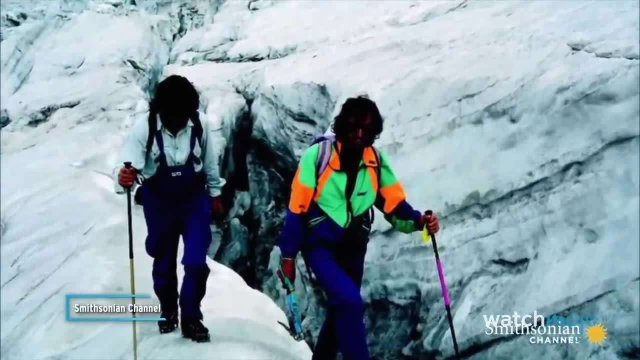 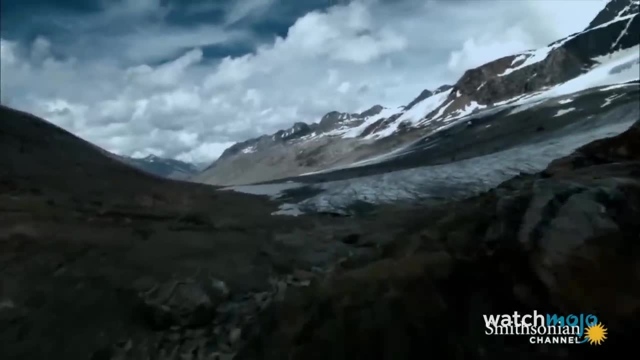 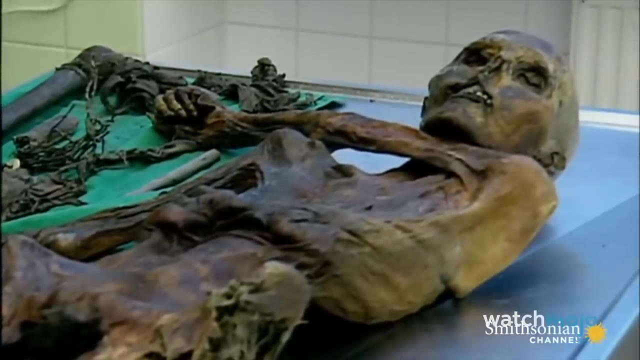 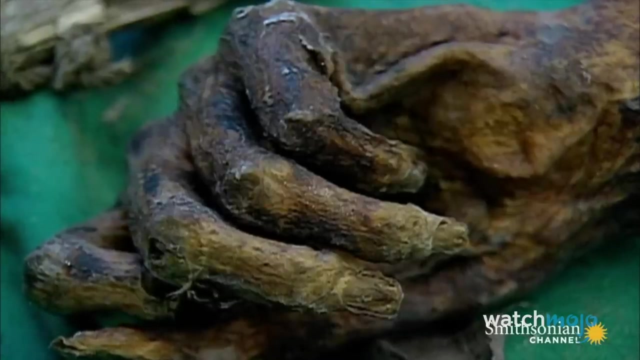 1991.. They found what is now known as Ötzi the Iceman, a natural mummy dating to about the 3230 BCE. Ötzi is the oldest natural mummy in European history, having died about 5,000 years. 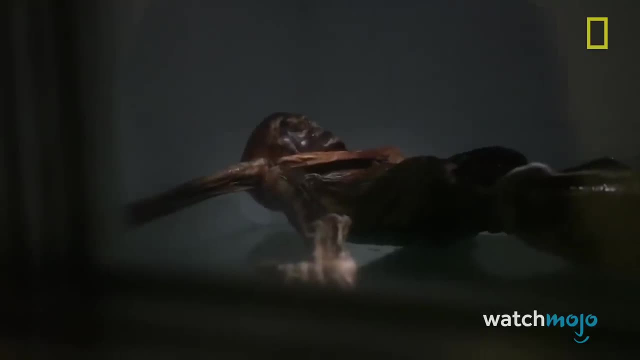 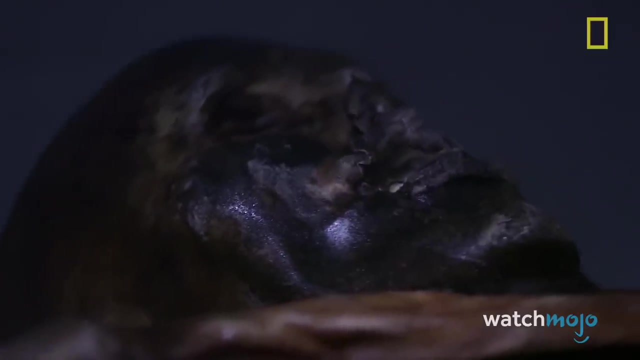 before he was found preserved in ice. Regardless, the body is in remarkable condition considering its age, and it's provided researchers an incredible glimpse into copper-age Europeans and their lifestyles. 17. The Serapium of Alexandria and the Serapium of Alexandria. 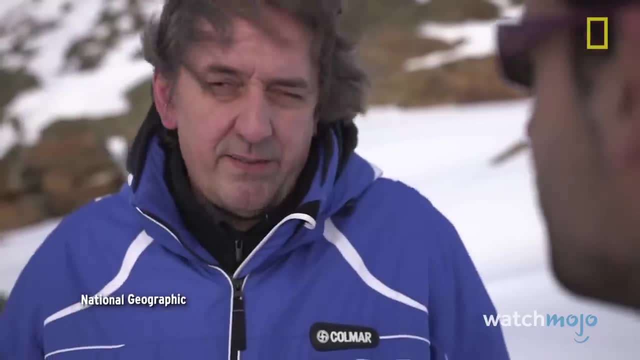 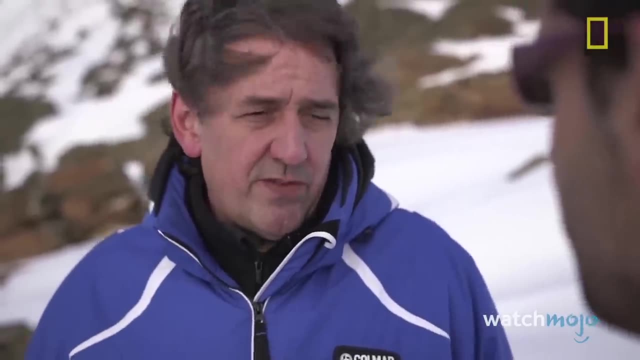 For sure. we want to know about how he died and why he died, because it's also such a spectacular finding This mummy, such an old mummy, is the only one we have here. 13. Mohenjo-Daro, A large human settlement dating. 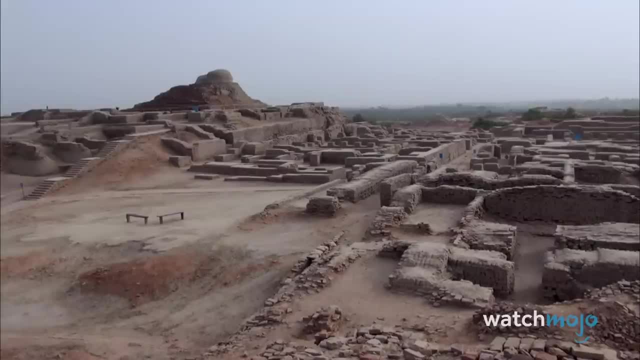 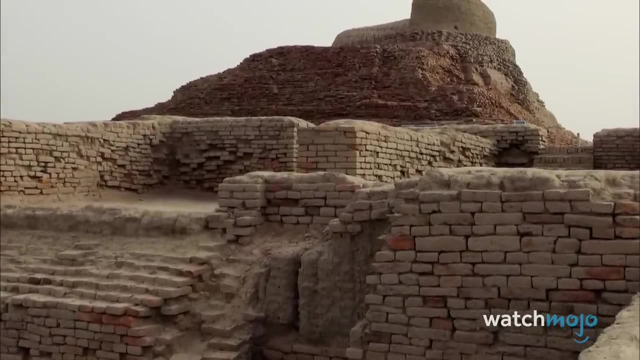 to 2500 BCE. Mohenjo-Daro is one of the oldest cities in the world. Located in modern-day Pakistan, Mohenjo-Daro was one of the most ambitious cities of its day, complete with street grids, a sewage system and many other ingenious feats of engineering. 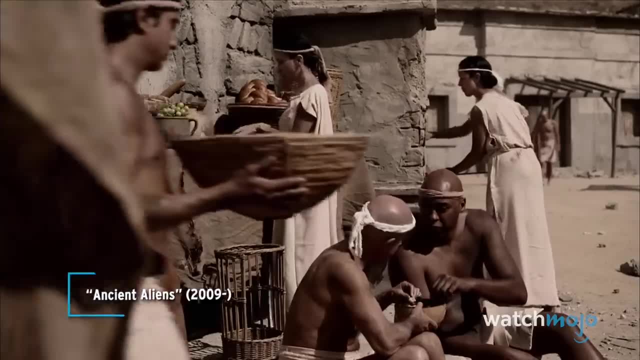 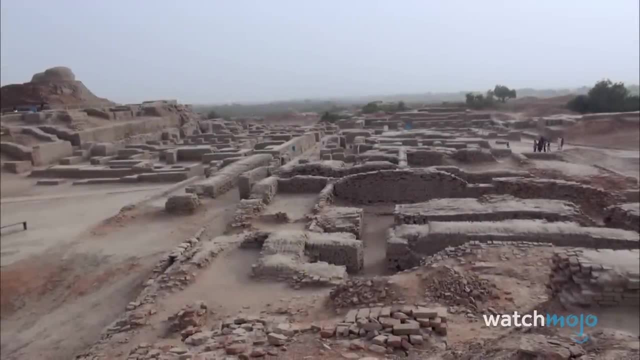 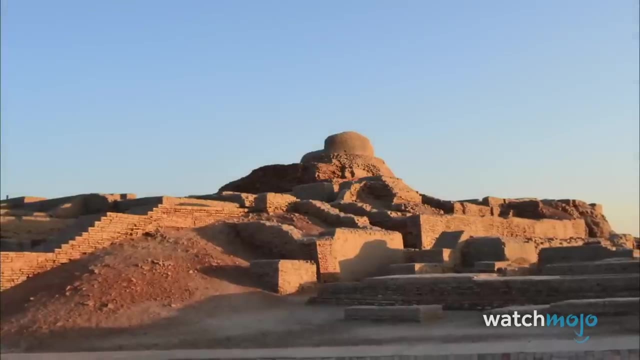 The city of Mohenjo-Daro rivaled the ancient civilizations in Egypt and Mesopotamia. Archaeologists believe that over 35,000 people once occupied the city. It was a remarkable settlement that showcased the creativity and boundless imagination of humanity. 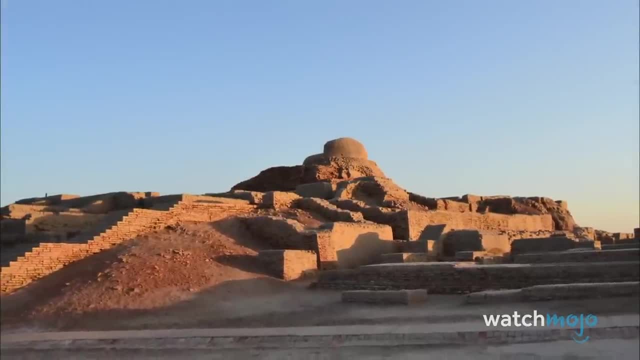 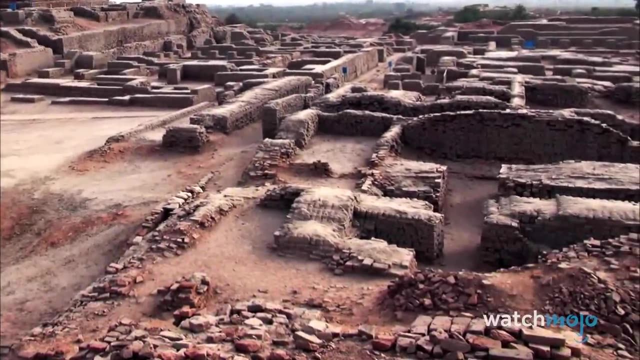 Unfortunately, Mohenjo-Daro was completely abandoned around 1900 BCE as the local Indus civilization went into a decline. It remained lost to time until the 1920s, when an officer of the Archaeological Survey of India located the ancient city. Sixty years after its discovery, Mohenjo-Daro was named a UNESCO World Heritage Site. So far, only 10% of the city has been unearthed. The authorities have stopped digging because they don't have the resources to preserve what has so far been discovered. 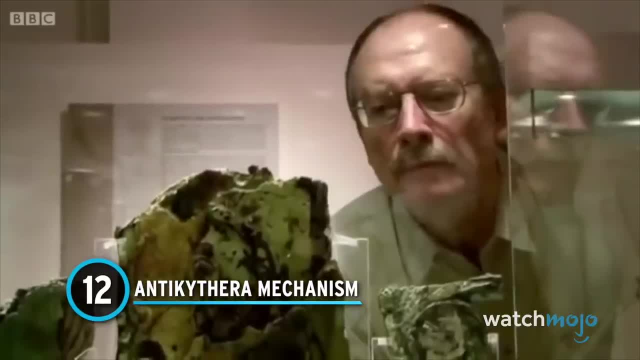 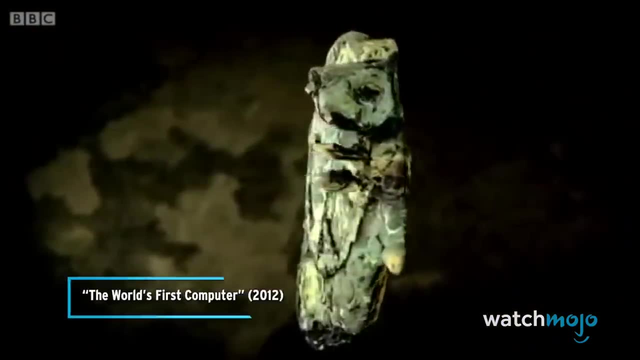 Number 12. The Antikythera Mechanism. If it hadn't been discovered when it was in 1901, no one would possibly believe that it could exist because it's so sophisticated. This mysterious object was found submerged in Grecian waters at the turn of the 20th century. 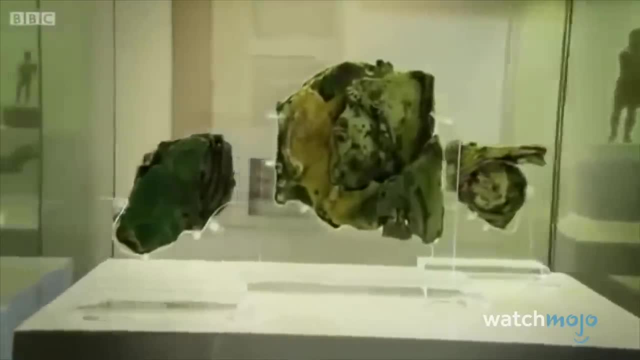 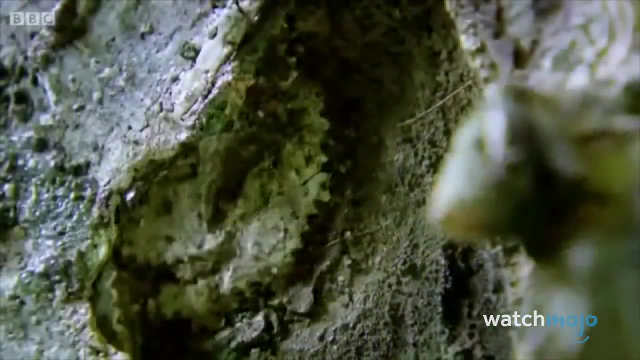 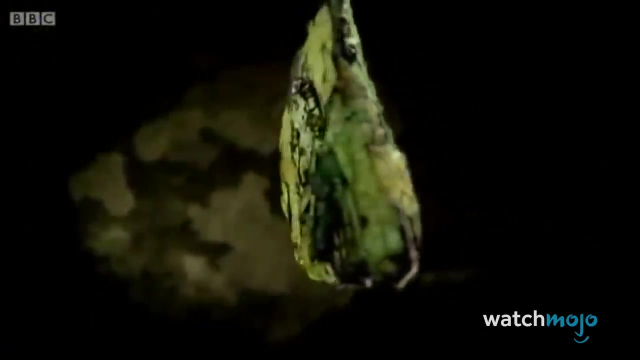 located inside an ancient shipwreck. The strange device was already 2,000 years old when it was found and, despite being eroded by the sea for all that time, it was still eventually identified as the world's oldest computer. Finally, another century after its discovery, and we now know definitively what it did. 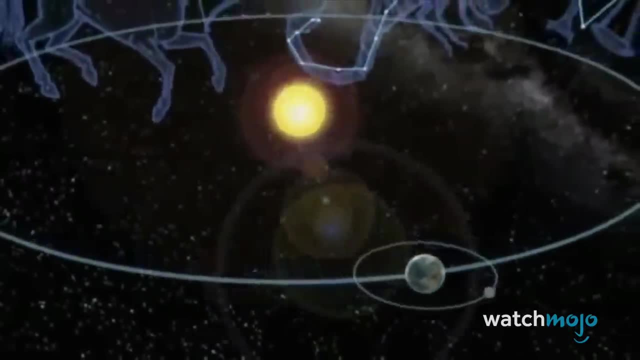 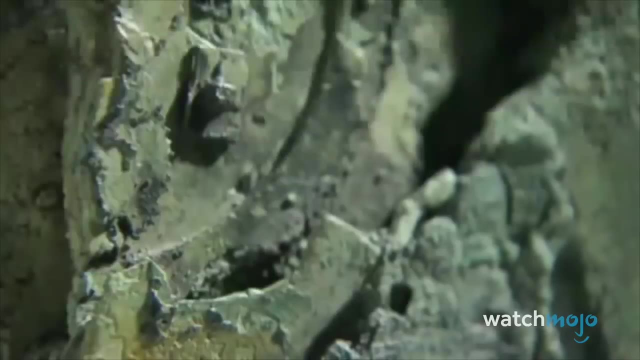 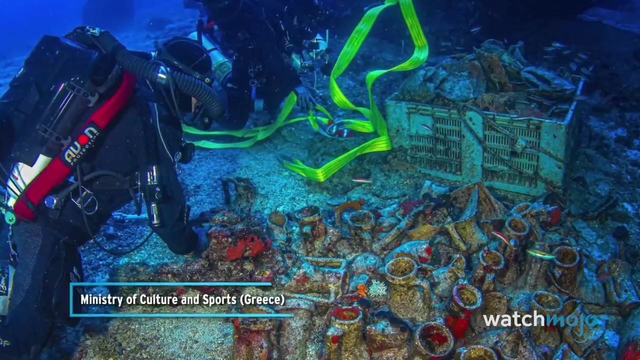 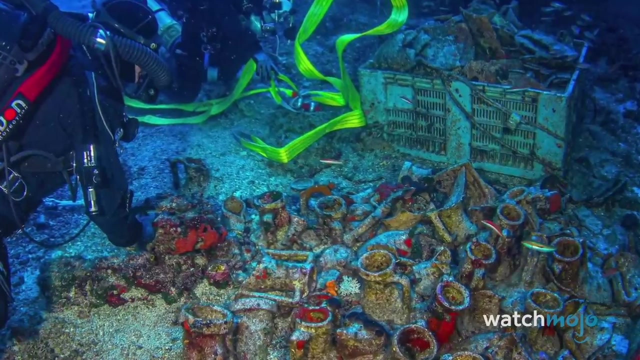 It was a device used to chart the positions of celestial bodies so that the ancient Greeks knew when eclipses would happen. It took a 3D reconstruction of the entire device in 2021 to get a better understanding of how it worked, though its purpose was suspected for decades. 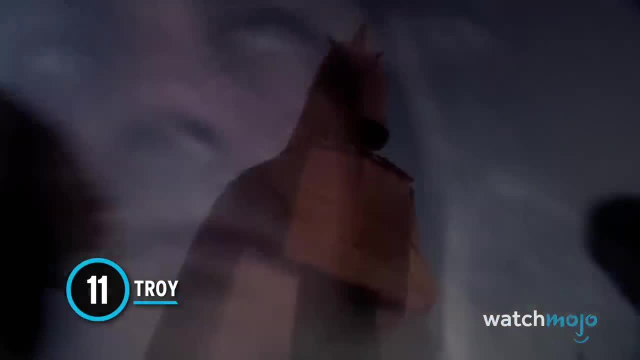 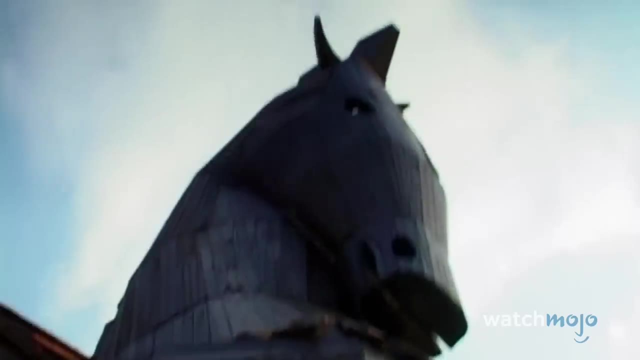 Number 11. Troy. For centuries, historians debated not only whether the Trojan War actually happened, but also whether the lost city of Troy ever existed at all. It's a story that's been told and retold by poets and actors for thousands of years. But is it real? Did the city of Troy actually exist? The Trojan War is the focus of one of ancient Greece's most famous epic poems, Homer's Iliad, and legendary Greek heroes like Achilles and Odysseus fought in it. 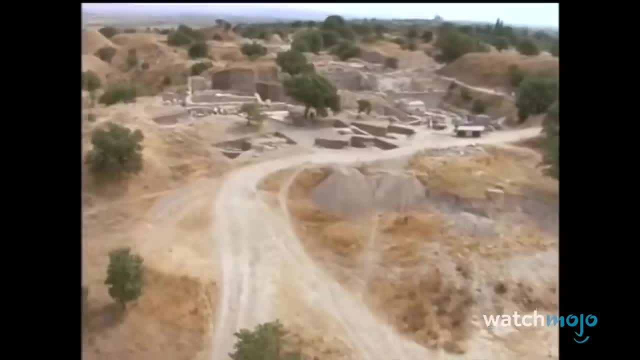 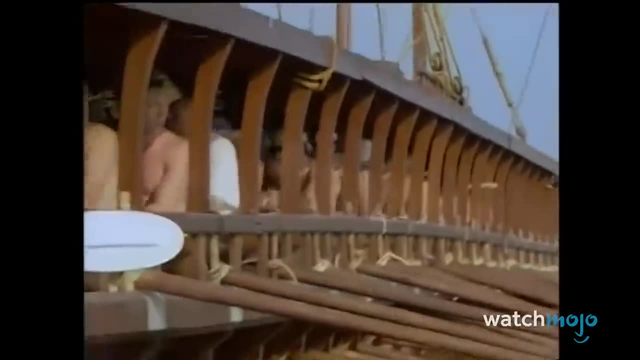 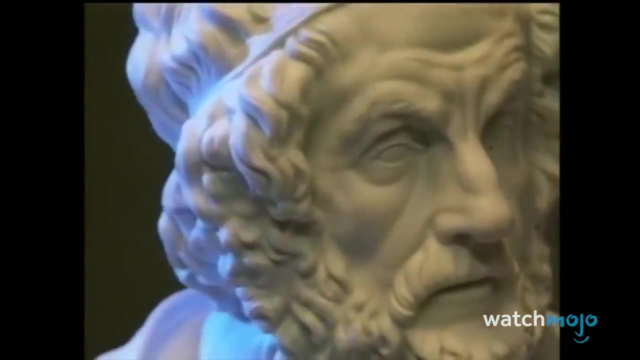 But Troy's location became lost knowledge. Throughout the 1800s, many researchers argued that Hisarlik, a site in western Turkey, was probably the elusive city. Throughout the 20th century, scholars have become aware that we can't even be sure that Troy is indeed this Troy. 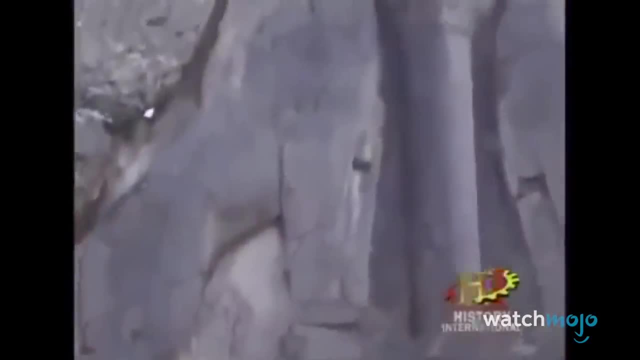 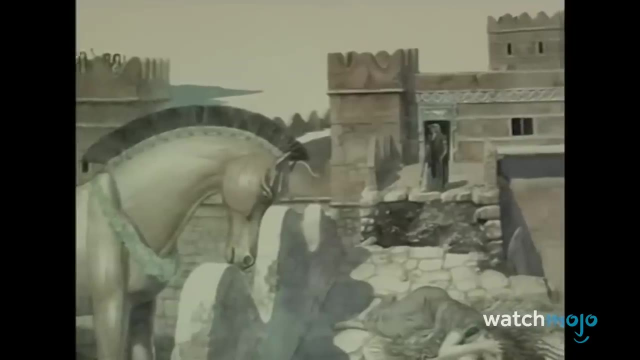 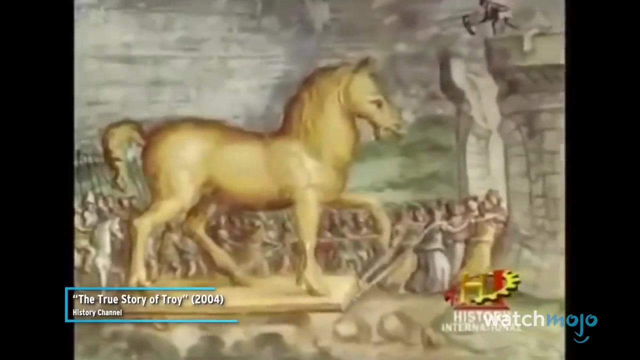 Finally, after decades of debate, experts came to a consensus that, yes, Hisarlik is in all likelihood Troy. Unfortunately, we've yet to find conclusive evidence that the Trojan horse existed, But Troy's identification was hugely important for historians: The idea that the Greeks would have in fact built a large wooden horse. 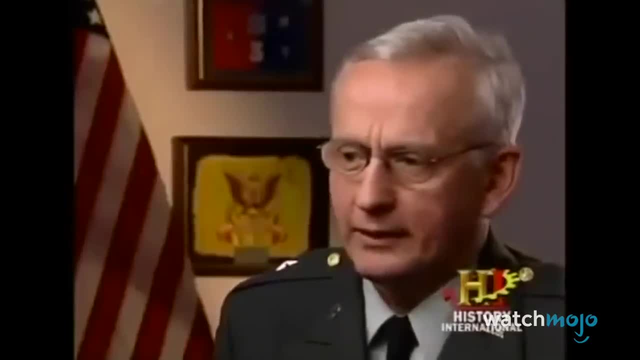 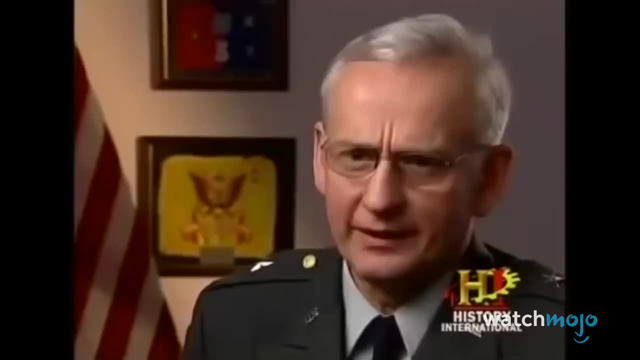 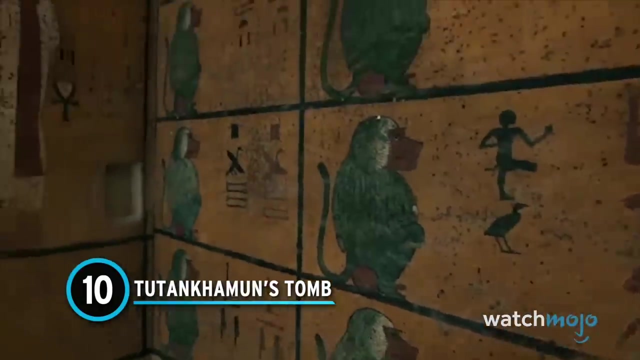 hidden inside it and had it dragged inside of. Troy is certainly possible, But it kind of strains your credulity a little bit that someone really could have pulled that off. Tutankhamun's burial chamber is filled with magical decoration, But beside it the rest of the tomb is left bare. 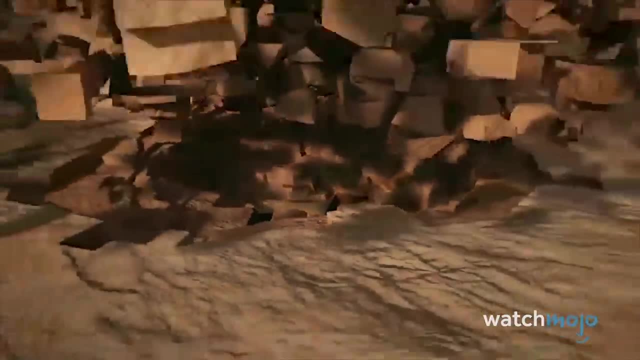 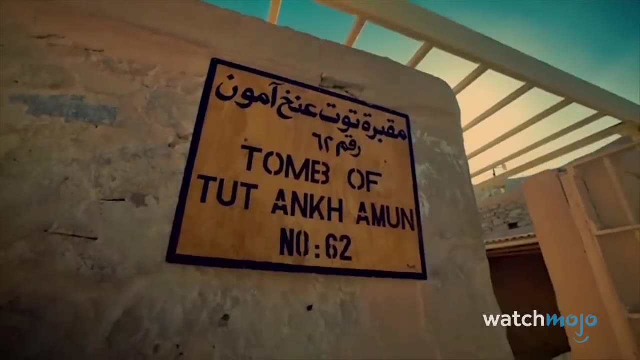 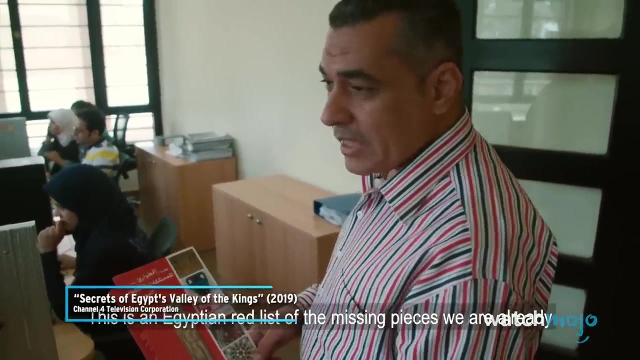 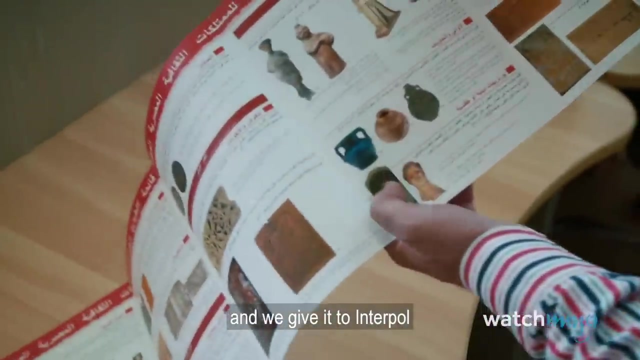 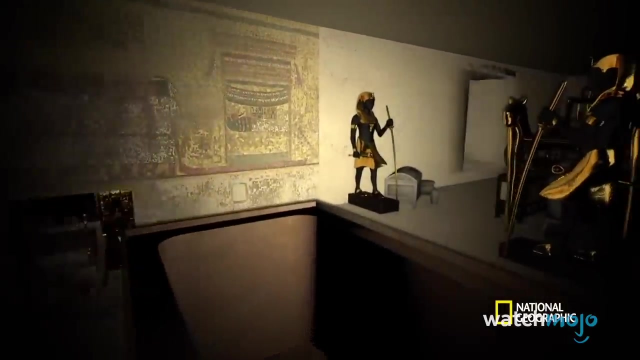 This simple tomb is unlike any other royal tomb in the valley. The Valley of the Kings is the final resting place of many ancient Egyptian pharaohs, But throughout its history, a number of tombs have fallen victim to grave robbers. Tutankhamun's tomb was different. Remarkably, though, grave robbers 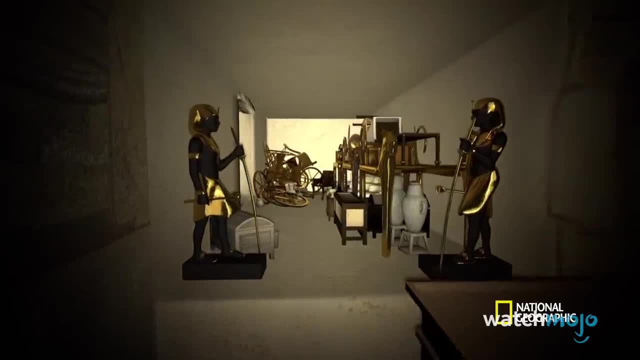 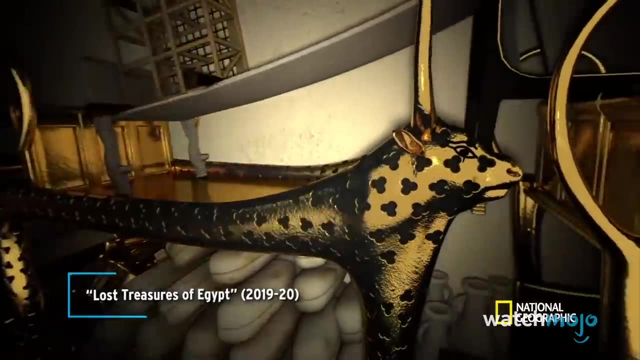 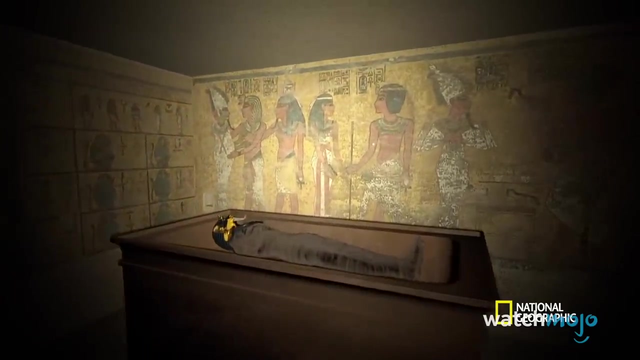 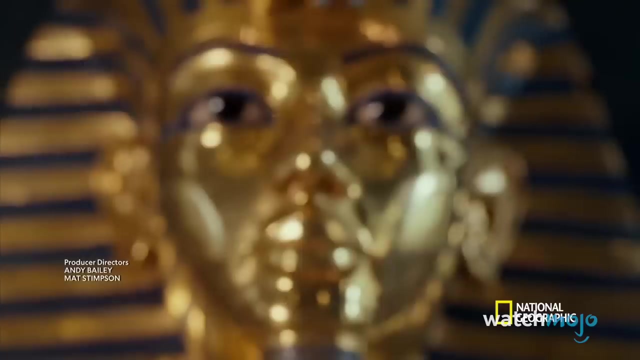 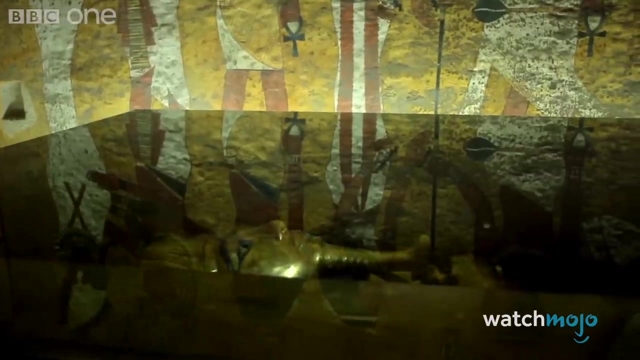 did break in shortly after it was initially sealed up. most of its contents were intact when archaeologists found it in 1922.. Today, Tutankhamun's gilded mask makes him arguably the most famous and recognizable pharaoh in history. Considering Tutankhamun only reigned for about ten years and died between the 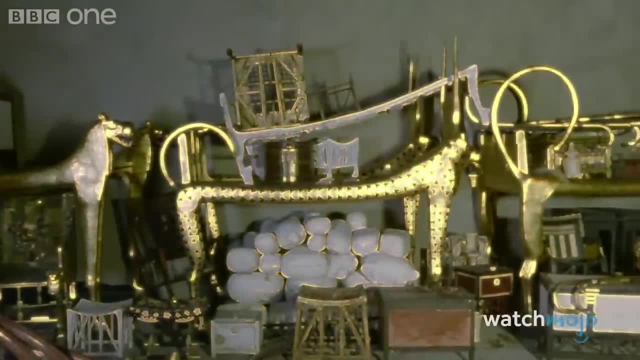 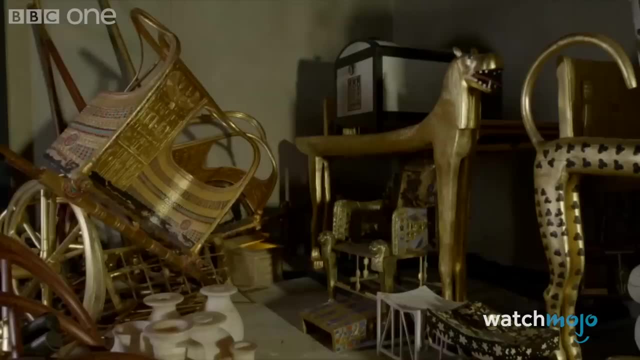 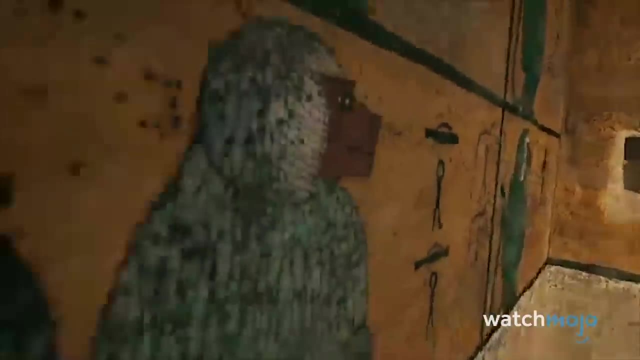 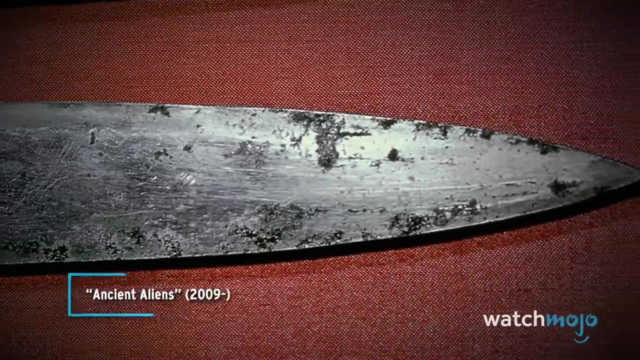 young ages of 18 and 19,. that is quite the legacy. Along with the mask, the tomb also contained a statue of Anubis, the god of the dead, and a dagger made from a fallen meteor. 9. Sutton Hoo, One of the most remarkable medieval graves. 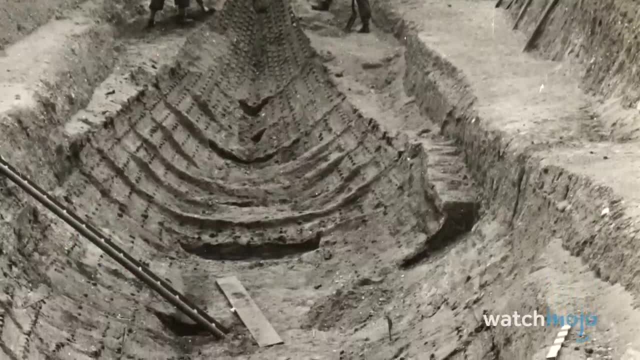 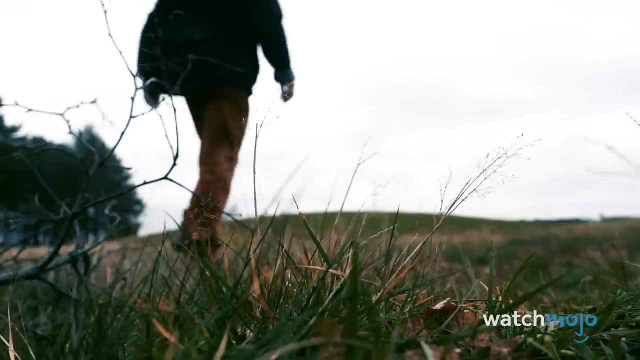 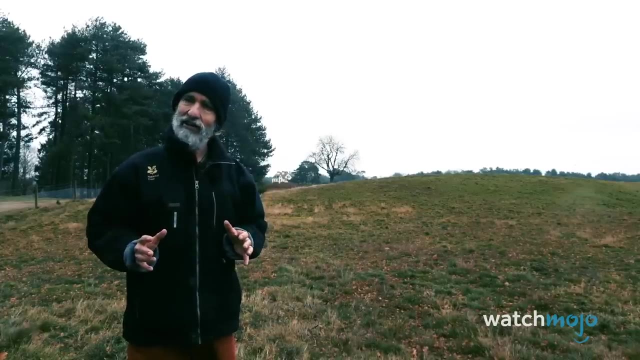 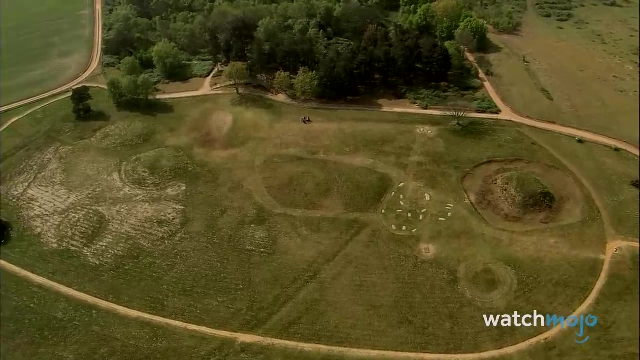 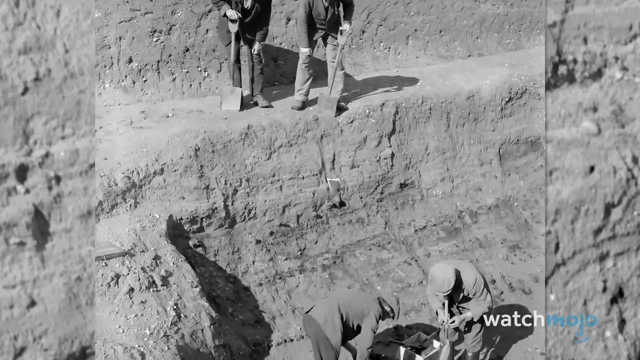 anywhere in Europe was excavated in England in 1939.. The owner of an estate in Suffolk, Edith Pretty, enlisted some archaeologists to find out what was underneath the burial mounds on her property. What they uncovered was astounding, So much so that the story inspired a 2021 film, The Dig. 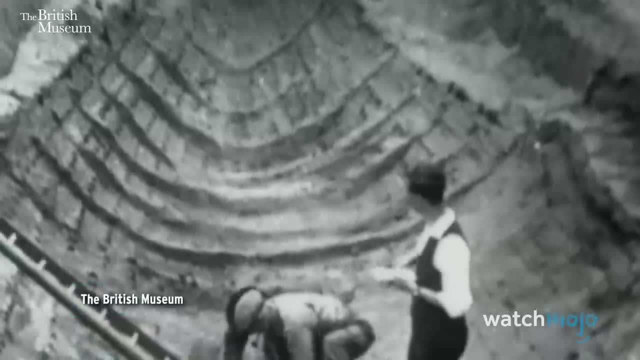 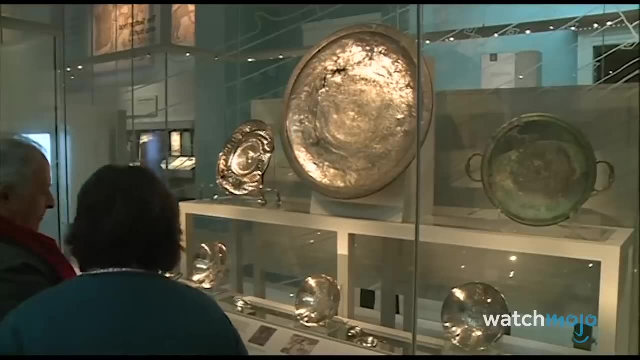 The most promising mound contained an entire long ship and innumerable artifacts, including pieces of armor made of gold and other Anglo-Saxon relics. Though it's one of the UK's most impressive archaeological discoveries, it's still not entirely clear whose grave it actually is. 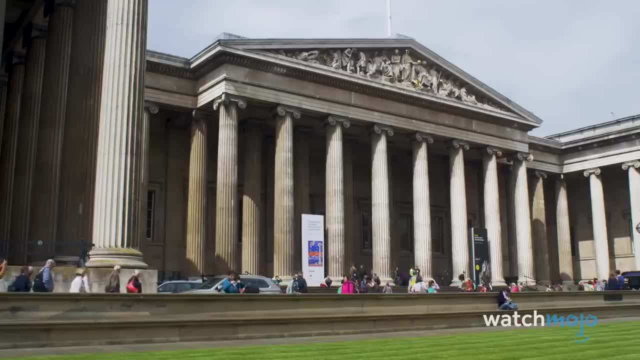 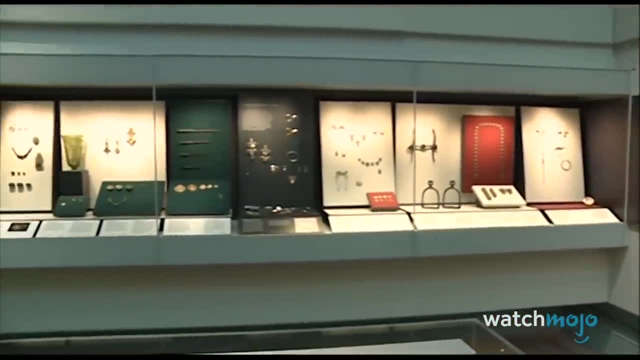 Shortly after the inquest, which ruled that all the items found in the Sutton Hoo burial mound lawfully belonged to Edith Pretty, Pretty donated the entire collection to the British Museum. It's among the most valuable donations of its kind and the collection itself remains at the heart of the museum. 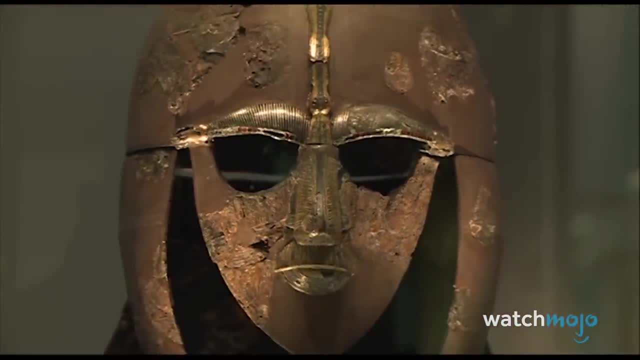 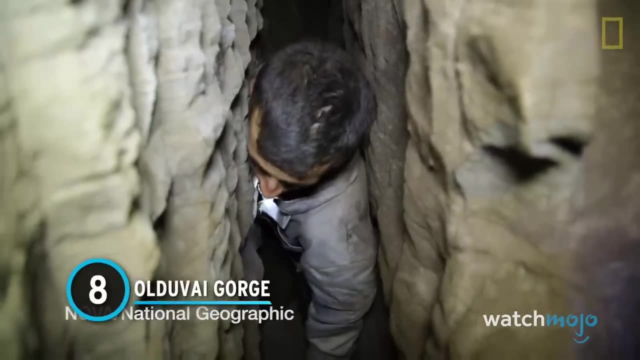 Most evidence suggests it was the final resting place of a famous East Anglian king, Redwald, who ruled the region around 1400 years ago. Number 8. Aldivai Gorge. This isn't one specific archaeological location but an entire locality housing some of the most. 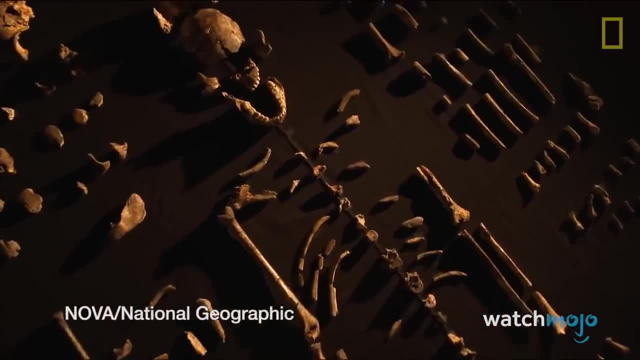 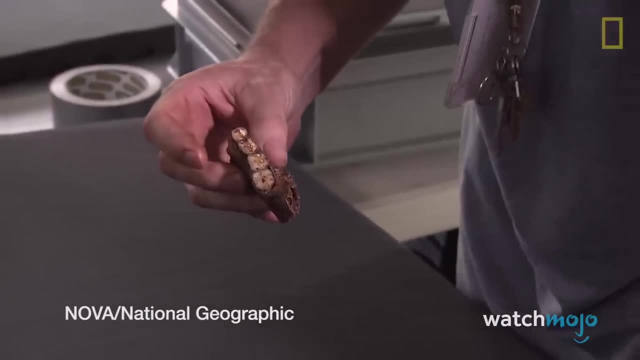 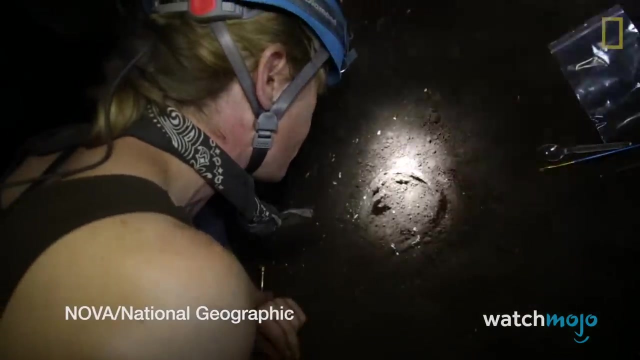 important works relating to paleoanthropology or the study of early humans Found in the northeast corner of Tanzania, Aldivai Gorge has been invaluable in our understanding of early human culture and evolution. Telling us is that there's a lot out there to be found. We actually don't have the whole story of. 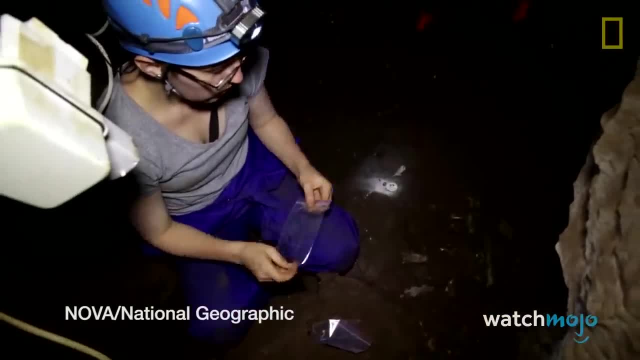 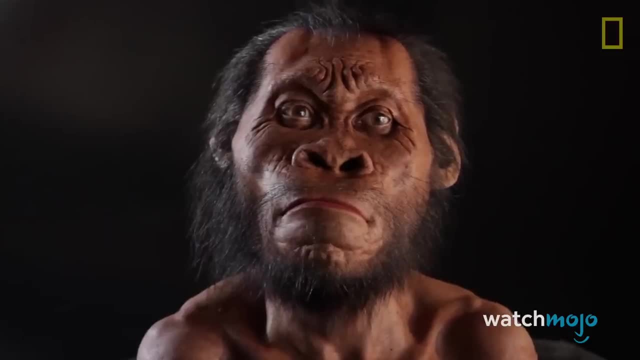 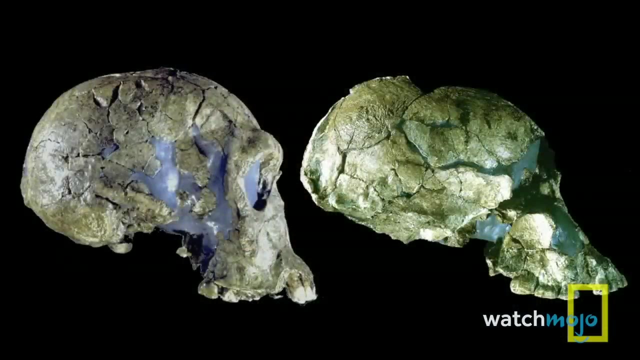 human evolution. Researchers have unearthed ancient stone tools and hominid fossils. Occupation of the site is believed to stretch back nearly two million years, when it was inhabited by an archaic human species called Homo habilis. And then these other things, which are generally termed Homo habilis after the. 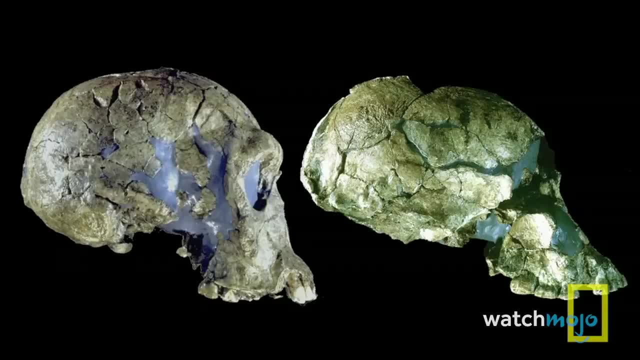 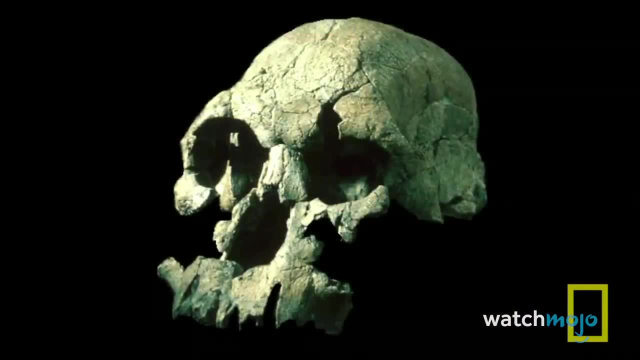 species that Lewis Leakey named at Aldivai in 1960.. Without Aldivai Gorge and its riches of archaeological material, our understanding of archaic humans would be much more limited. Number 7. The Cave of Altamira. 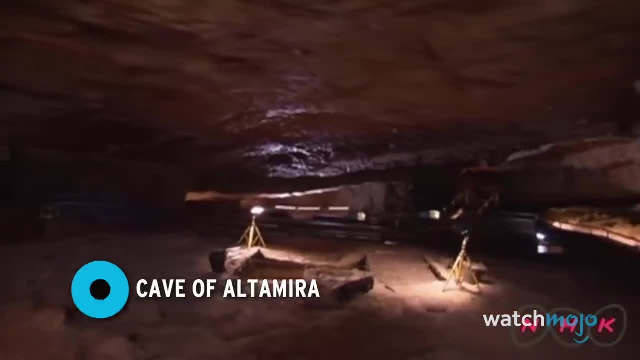 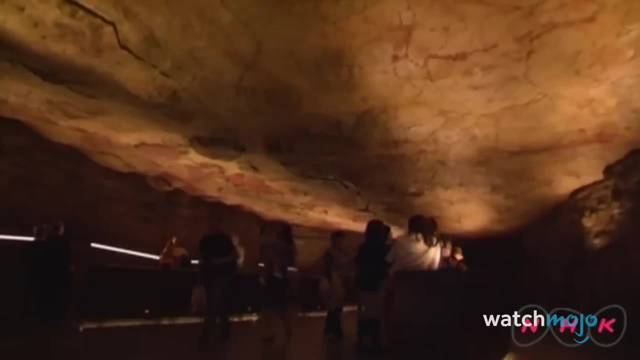 If you're interested in early humanity, then you cannot go wrong with the Cave of Altamira. This is the Museum of Altamira. It was built right next to the cave where the original cave paintings dating back to the Paleolithic era were discovered. 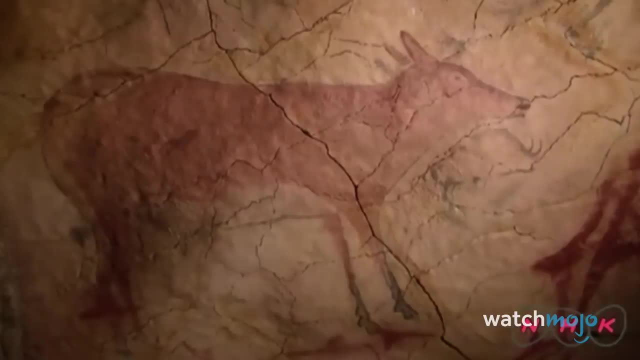 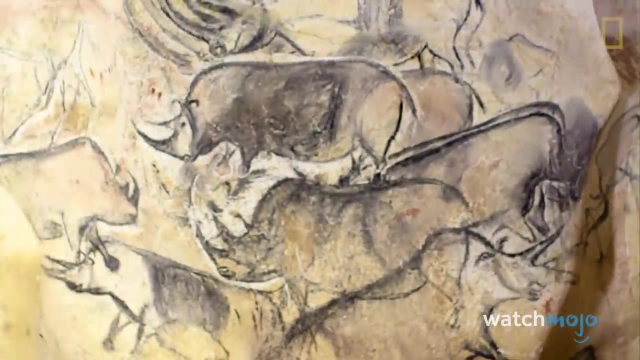 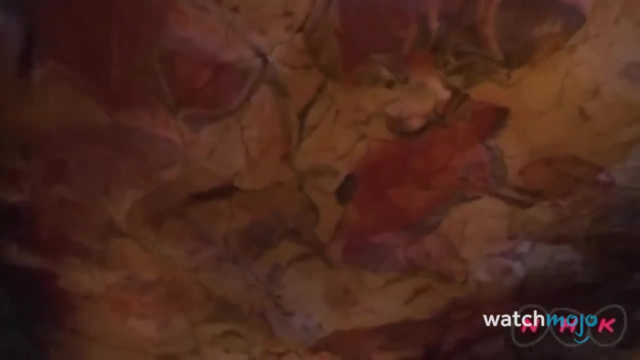 The original cave has been closed to preserve its archaeologically important remains. Archaeology has uncovered many notable caves relating to ancient humanity, Including Lascaux and another in the small Spanish town of Artales, But nothing beats Altamira, Also located in Spain. this cave houses numerous prehistoric drawings and paintings. 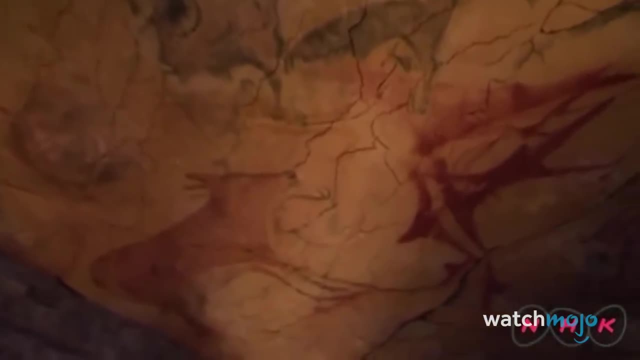 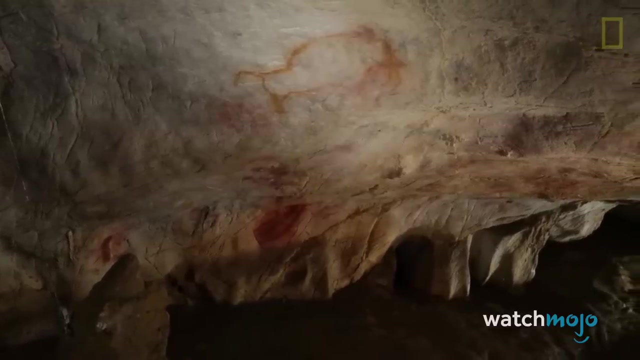 most of which depict local animals. After the site was discovered in 1868, the suggestion that the paintings were prehistoric was met with some skepticism, Not only owing to the nature of the drawings, but also because no other prehistoric cave art was known to exist in Europe. 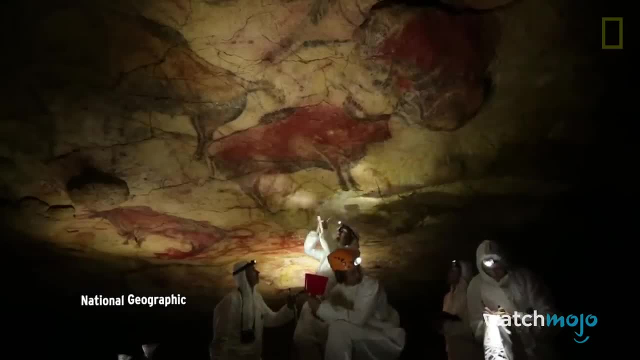 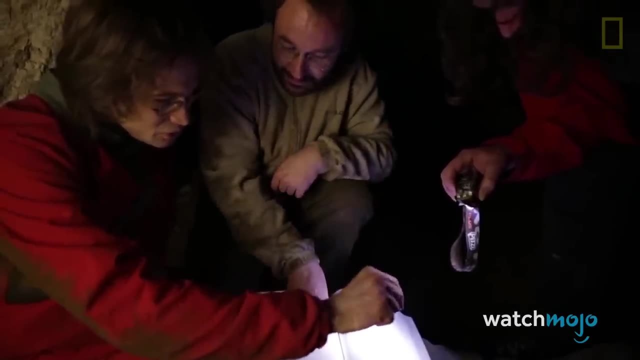 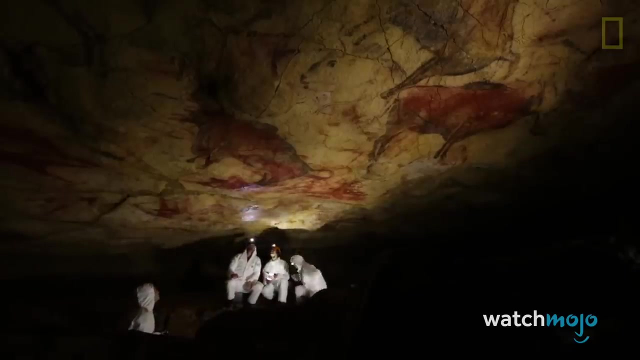 We're also interested in in whether or not human symbolic behavior coincides, for example, with language, or whether human symbolic behavior in fact dates right back to the point at which we start looking like humans. But the research eventually prevailed and it's now believed that the paintings are around 36,000 years old. 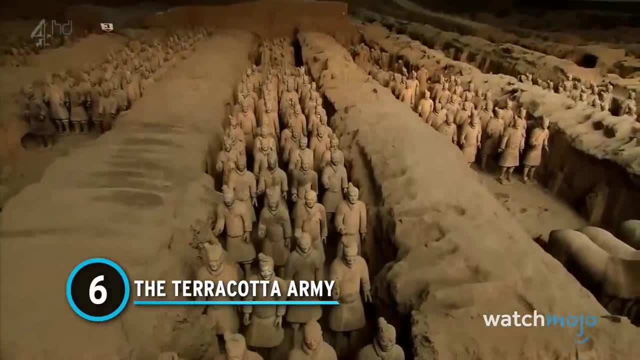 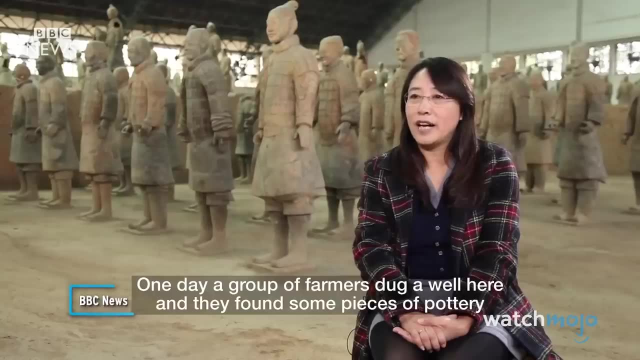 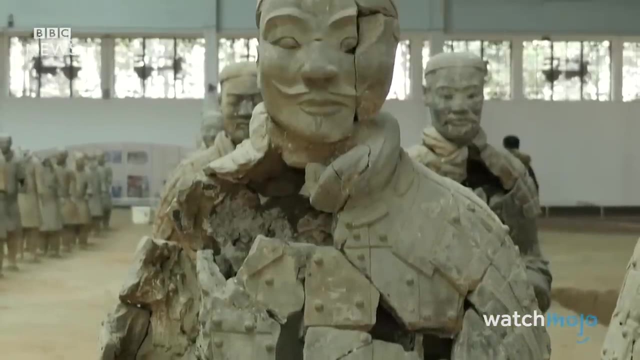 Number 6. The Terracotta Army. This is one of the most significant archaeological finds of all time and it was discovered completely by accident, And they find some pieces of the pottery. They also find the head of the terracotta warriors. 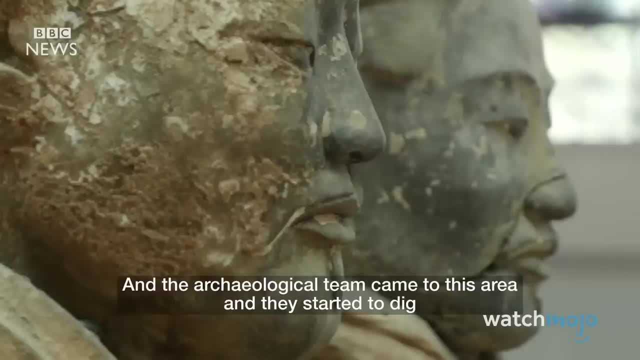 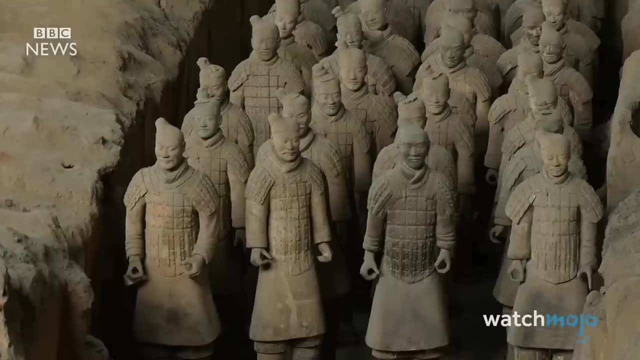 and the team archaeological team came to this area and they start to dig. The Terracotta Army was first uncovered in the Shanxi province of western China by a group of farmers in the 1970s. The army resides within a tomb constructed over 2,200 years ago. 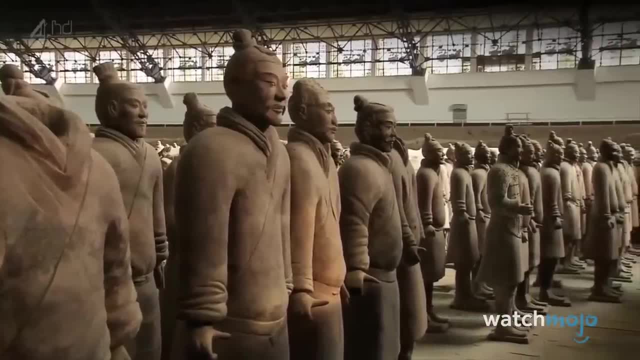 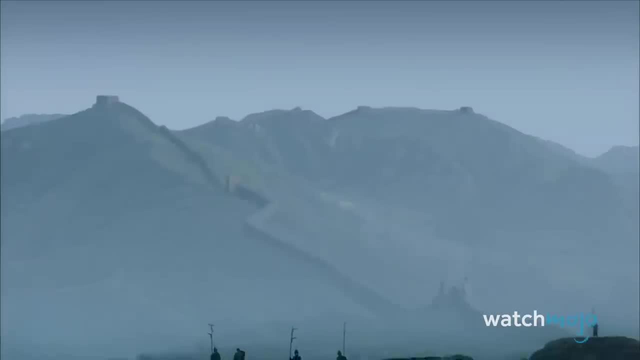 as the rest of the Terracotta Army. It's the resting place of Qin Shi Huang, the first emperor of China, which is why it's so elaborate. He was its first emperor, and his empire became his fortress, protected by a great wall. 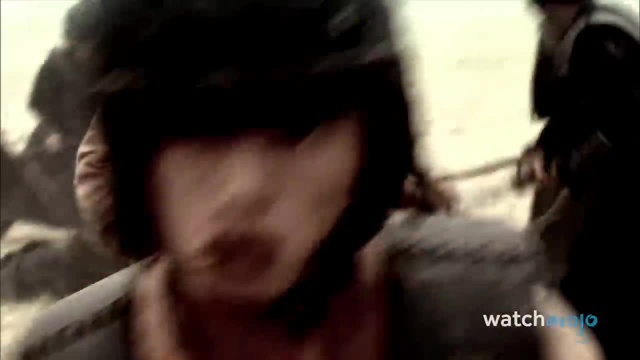 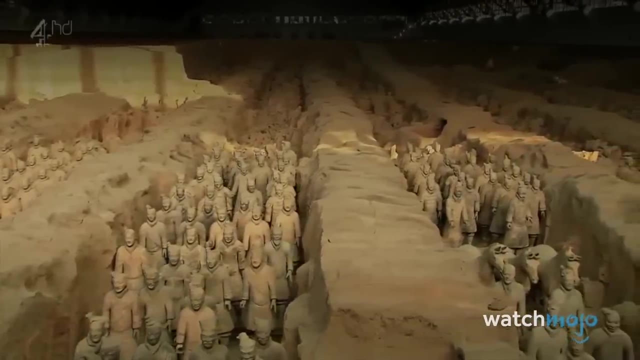 The legend says he was a tyrant driven mad by power. In the parts we've been able to excavate there are over 8,000 soldiers made out of clay there to guard Emperor Qin in the afterlife, Row upon row. hundreds of warriors, hundreds of secret subterranean soldiers, all life-sized and built to be immortal. But even more astonishing is the fact that the entire necropolis is believed to be almost 40 square miles in size, with most of the site hidden in vaults that aren't yet accessible. 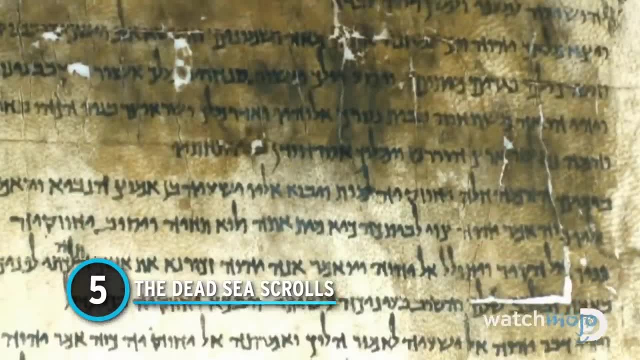 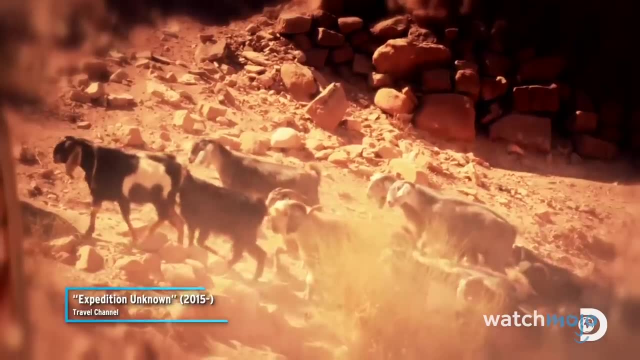 Number 5. The Dead Sea Scrolls, Written mostly in Hebrew, the Dead Sea Scrolls are some of the oldest Abrahamic religious texts in existence. A young shepherd is herding goats in Qumran, near the Dead Sea, Passing a cave. 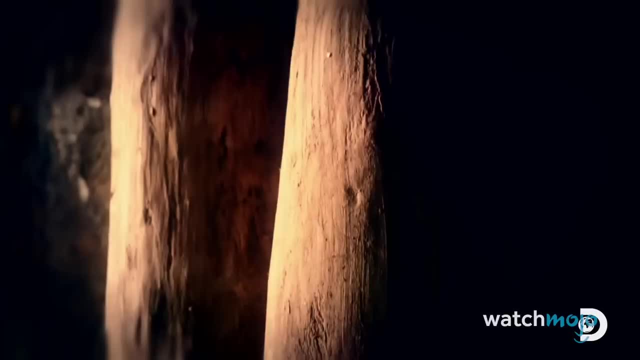 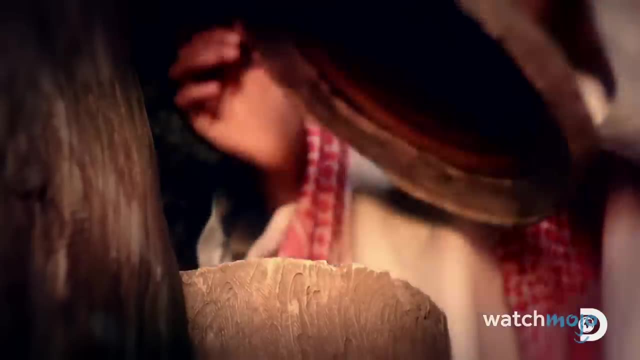 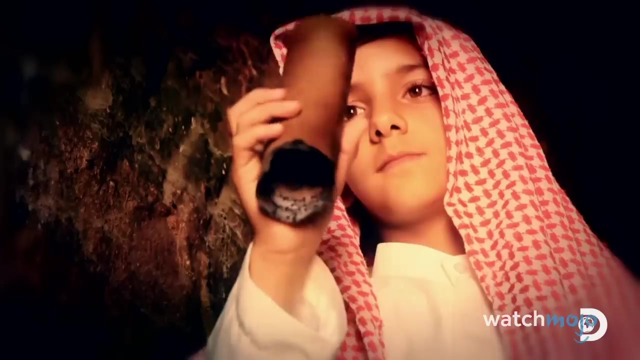 he throws a stone to scare a wayward animal back to the flock and hears something shatter Curious. he enters the cavern and discovers ten clay jars holding seven ancient scrolls. They were discovered in a cave in the West Bank in the mid-1940s. 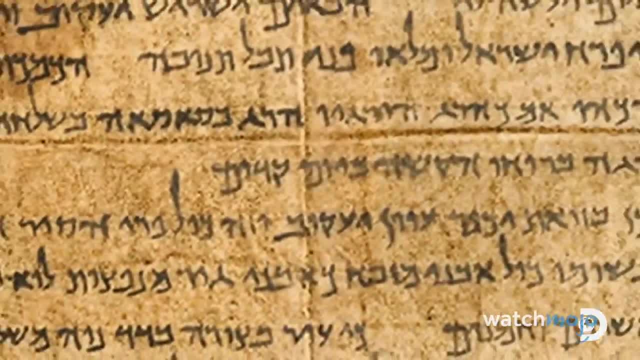 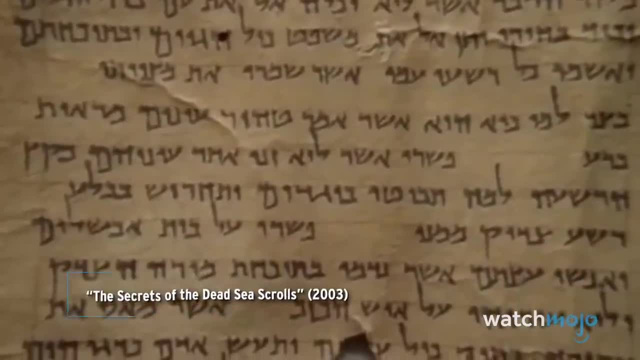 but in the decades since, we've continually found more and more scrolls ready to be translated in a handful of additional caves. The scrolls themselves talk of the battles of the great teacher of righteousness, who led the community into the wilderness, with the teacher of lies. 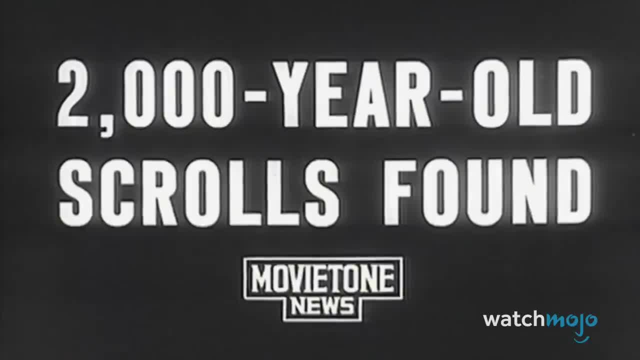 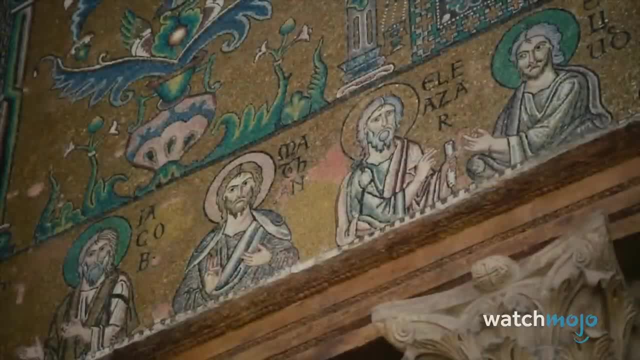 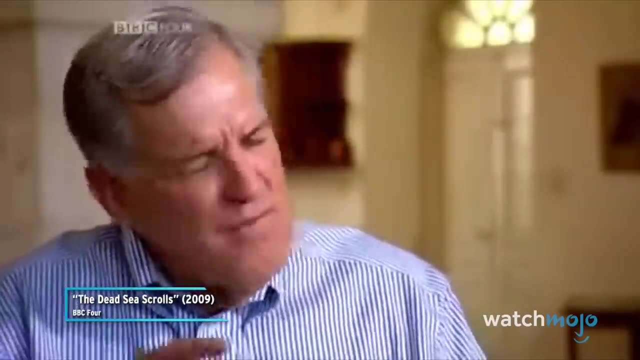 The scrolls are so significant because they've allowed historians and theologians to chart the development of the Bible much more accurately and provided new information about the dawn of Christianity thousands of years ago, as well as the history of Judaism and the Holy Land. Now we're becoming much more attuned to how very Jewish 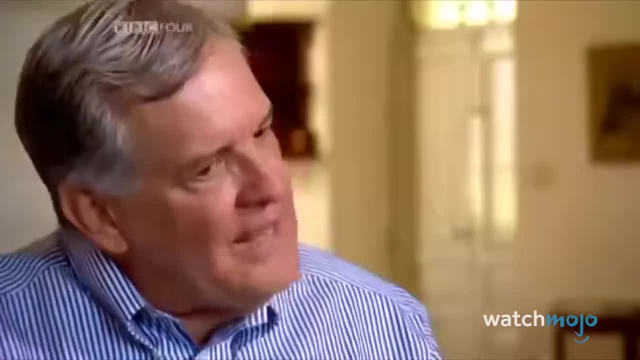 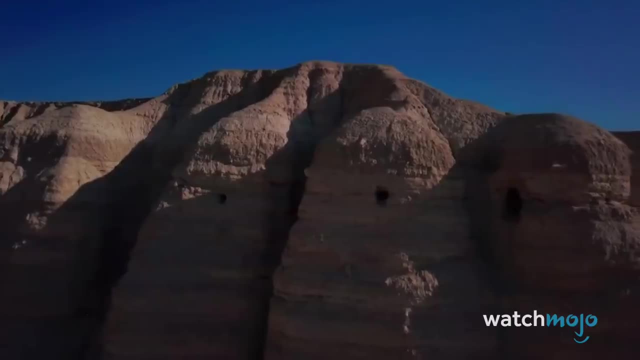 Jewish. Jesus was Very devout Jew, and that's the heart of Christianity. They are unquantifiably important and still have a lot to teach us. There's really no way of predicting what the next discovery is going to be or what it's going to come from. 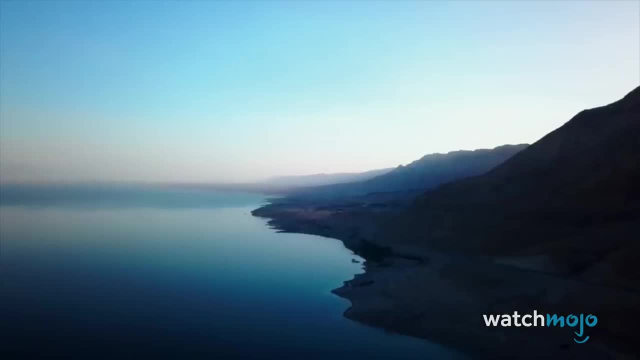 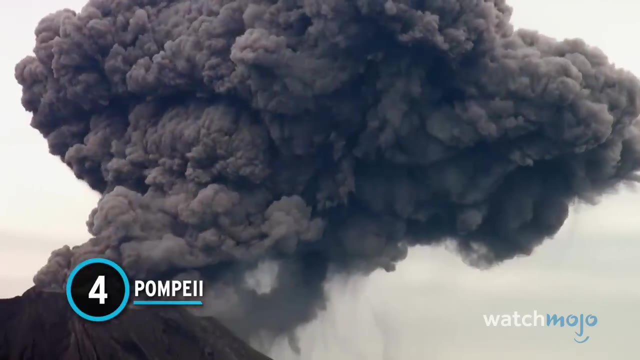 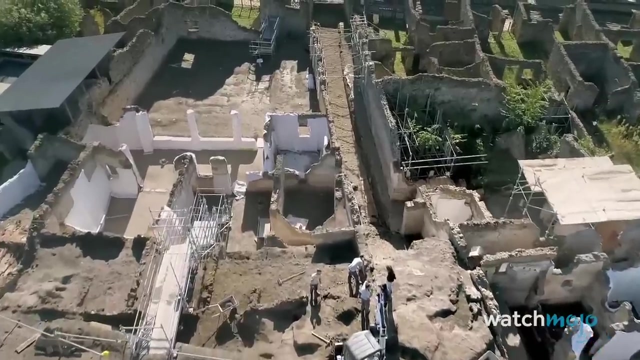 I think it's fairly reasonable to guess there will be something. Surely there will be something. Among the most famous ruins in the world, Pompeii was destroyed by a devastating eruption from Mount Vesuvius in the year 79, The village was left forgotten until the 16th century. 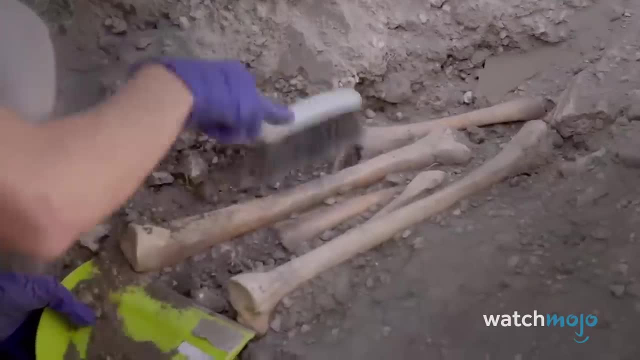 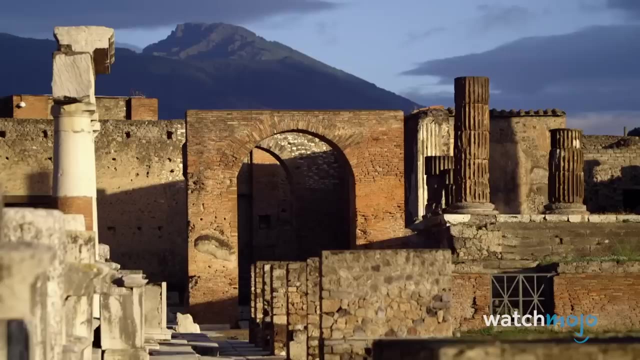 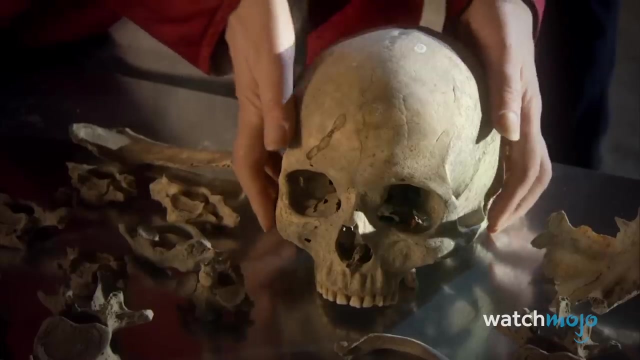 over 1500 years later, because it had been completely buried underneath volcanic ash. It took just 18 hours for Pompeii to be buried under millions of tons of volcanic ash and pumice. An entire living city wiped out, But that ash kept Pompeii largely intact when it was finally excavated. 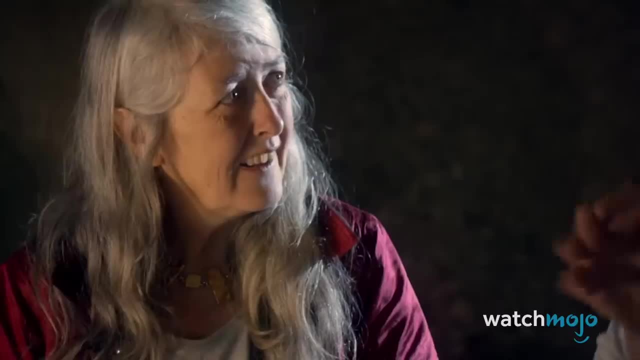 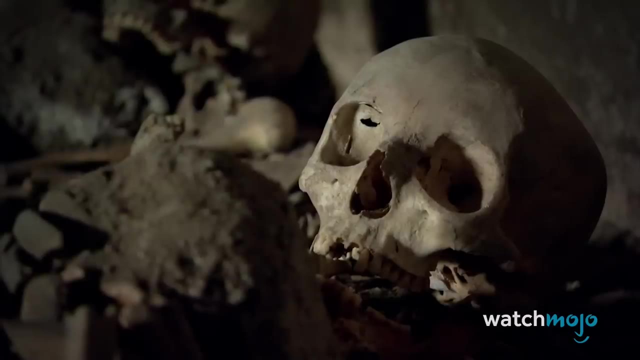 with people frozen in place where they died during the disaster. The point is, we have a great opportunity here because we have a snapshot of the society. We might have slaves, we might have upper-class people and we can find out if there have been big differences. 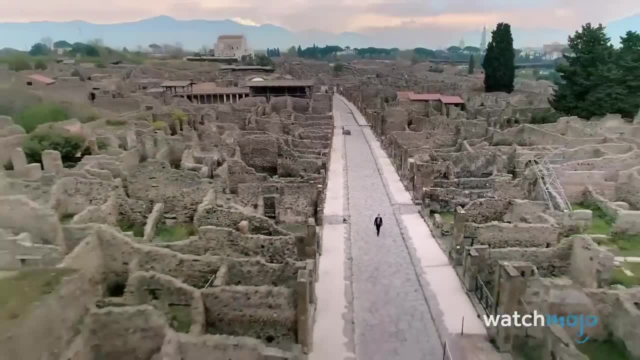 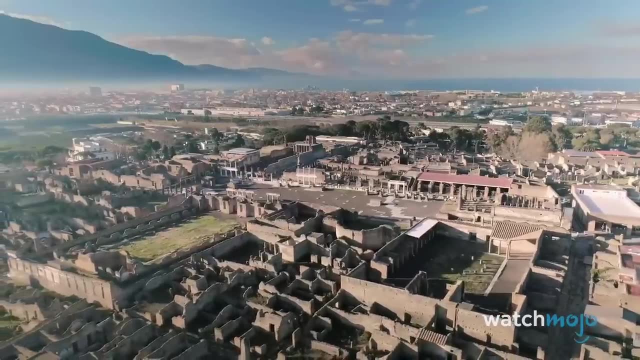 Today, it's one of Italy's most popular tourist attractions and a tremendous source of Roman history. As tragic as the story is, Pompeii has taught us more about Roman life than many other ancient archaeology sites anywhere in the world. Pompeii has regained its pride. 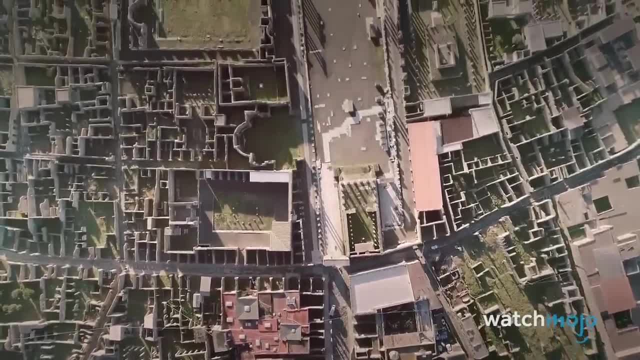 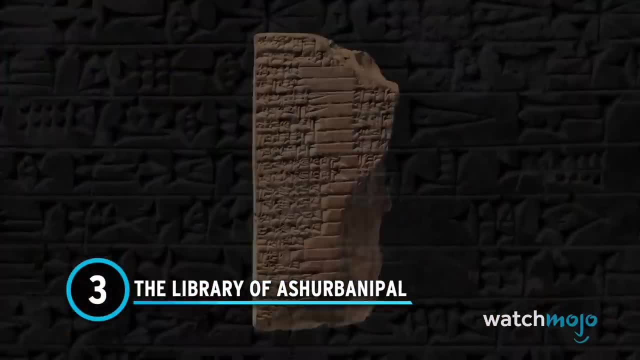 and continues to share its stories with people from all around the world. Number 3. The Library of Ashurbanipal. Famous writer HG Wells once called the Library of Ashurbanipal- quote- the most precious source of historical material in the world. And he wasn't far off. English historian and traveler Austin Henry Layard found the ancient library in the remains of a palace in 1849. While the actual building had been destroyed, many of the library's old texts were still intact, though most were in fragments. 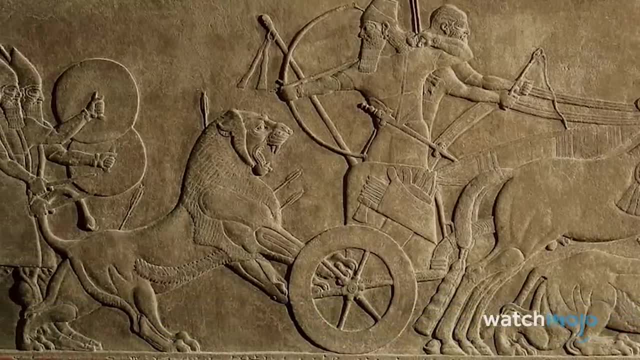 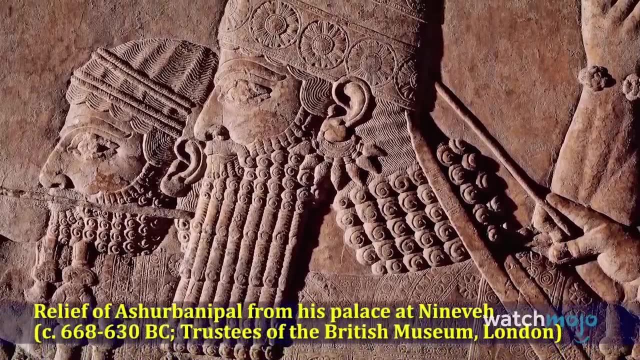 It consisted of over 30,000 clay tablets, which provided an enormous wealth of information relating to ancient civilizations of the Middle East. The tablets date to the 7th century BCE. Perhaps the greatest find within the Library of Ashurbanipal was the Epic of Gilgamesh. 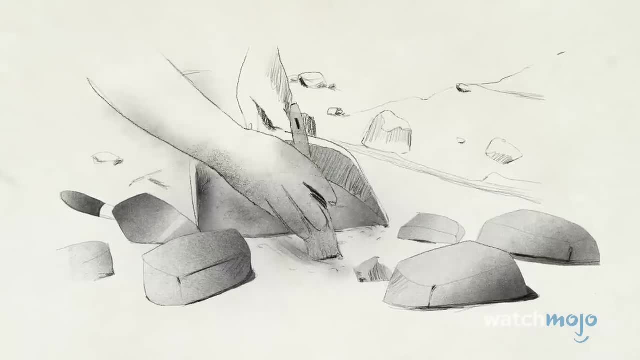 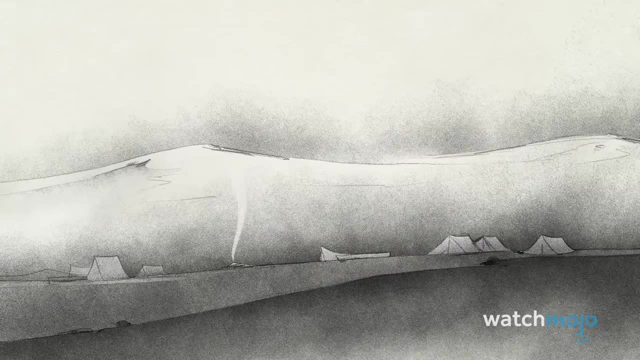 which is widely considered to be the oldest piece of literature in human history. Inscribed on crumbling clay tablets, was a 4,000-year-old story So riveting The first person to know that to translate it started stripping from excitement. 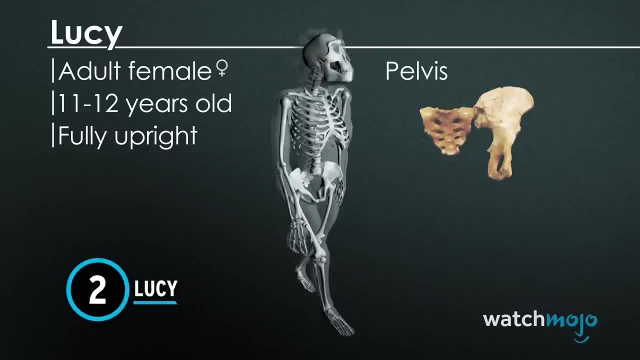 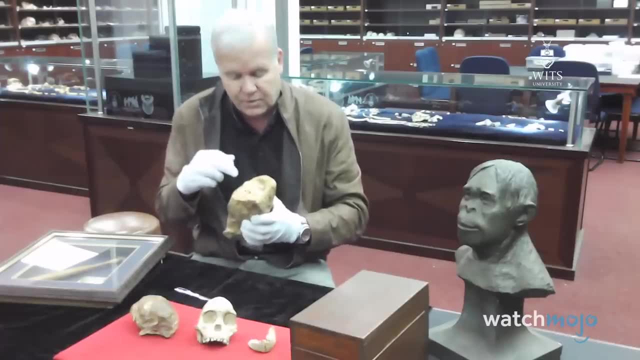 Number 2. Lucy. Several famous fossils have revolutionized our view of early hominins. Discovered in 1924 in South Africa, the Tong child, a skull of an Australopithecus africanus, was described as- quote- the missing link between ape and human. 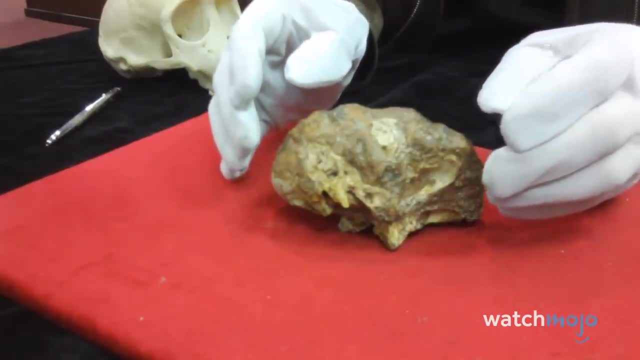 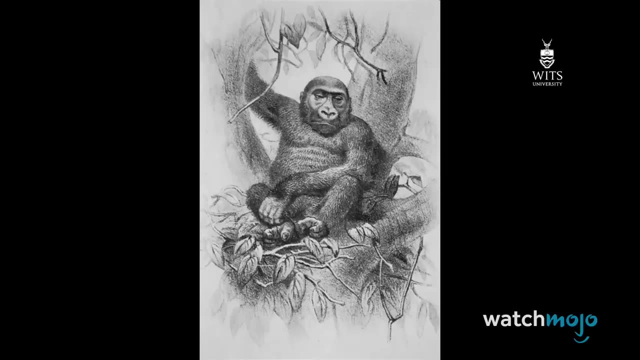 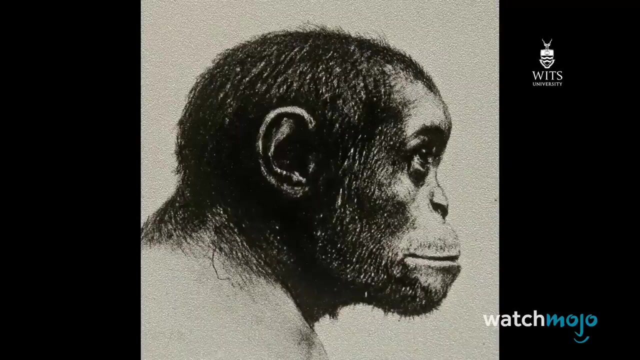 Although anthropologists initially resisted the idea that humans had evolved in Africa, Some scientists even went so far as to suggest it was perhaps just a baby gorilla and that the Tong child would bear little out on anything other than the origins of apes themselves. 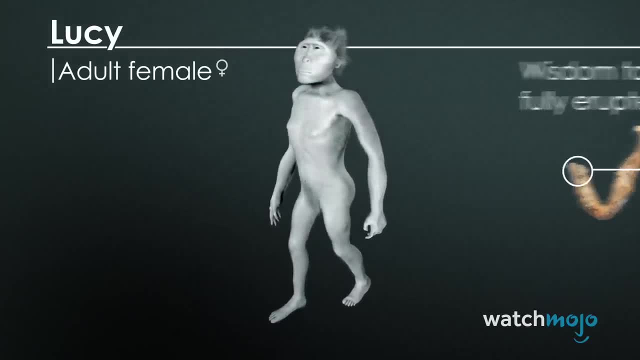 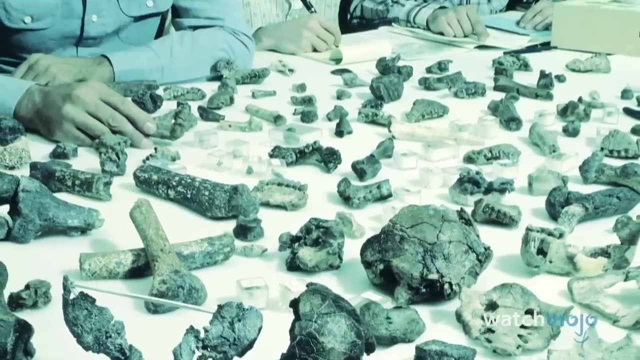 Eclipsing the Tong child in renown is Lucy, the 3.2 million-year-old remains of an Australopithecus afarensis Unearthed in 1974 in Ethiopia. she was named after the Beatles' song Lucy in the Sky with Diamonds. 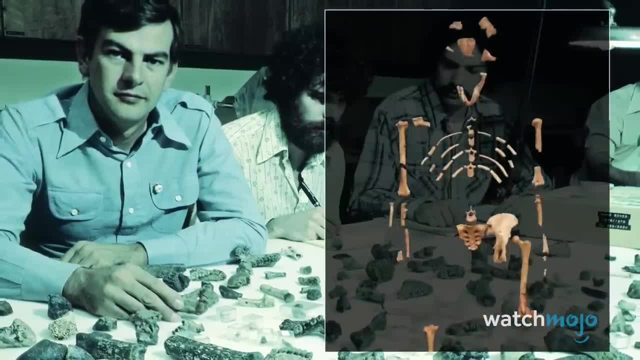 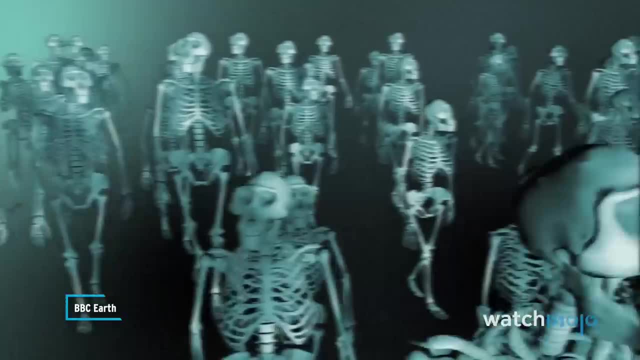 which the research team was playing on repeat. The completeness of her remains gave us much more information on the evolution of bipedalism and brain size. We now have 400 specimens of Lucy's species, Australopithecus afarensis. 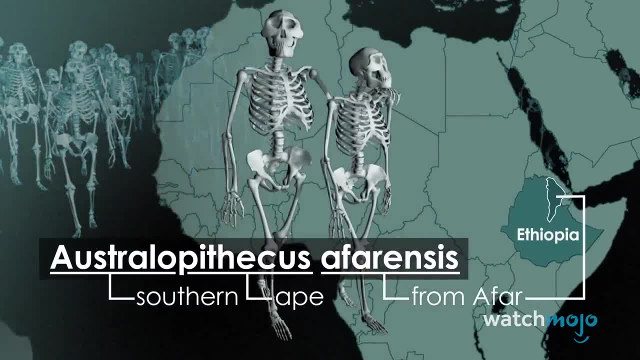 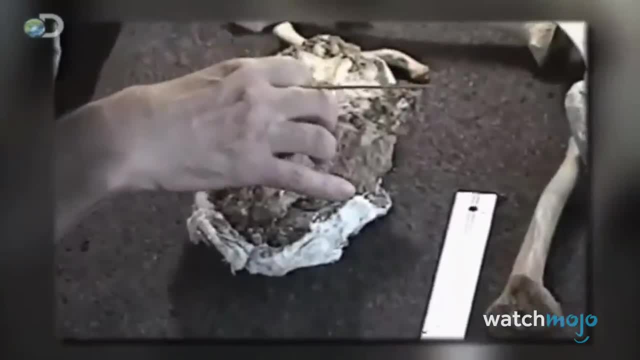 named after the Afar region and we know that there are very large individuals which were males and the smaller ones are certainly females. In 1994, Ardi, the skeleton of an Ardipithecus ramidus, thought to be 4.4 million years old.